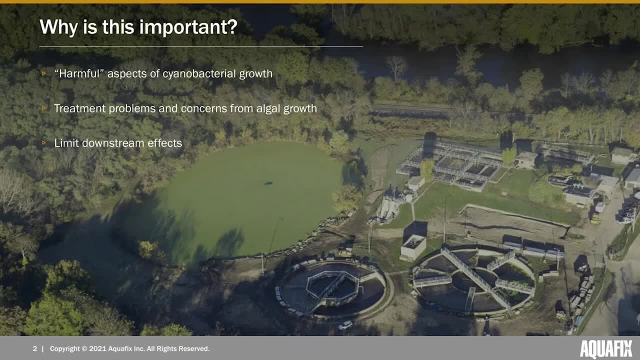 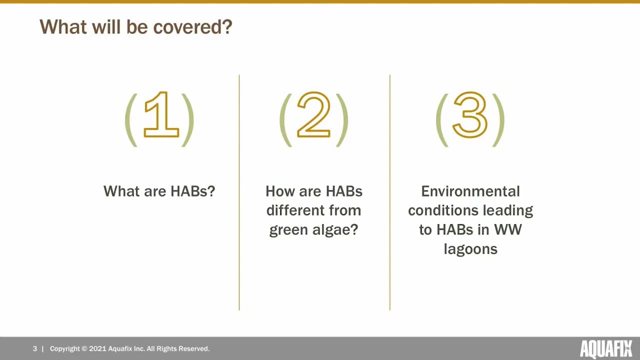 I want to highlight the downstream effects and the ways that we can prevent and limit these negative downstream effects from occurring due to the presence of HABs within a lagoon. So to outline today's presentation, first we are going to dive into HABs and answer the question of what exactly? 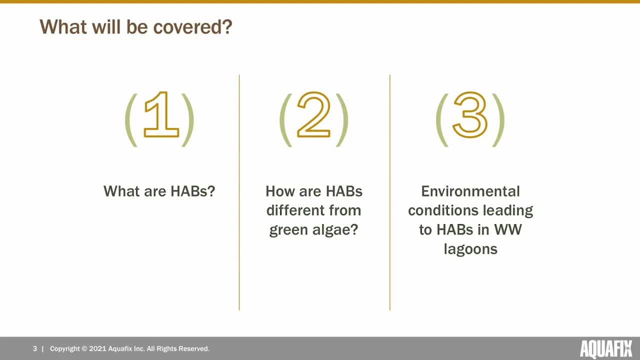 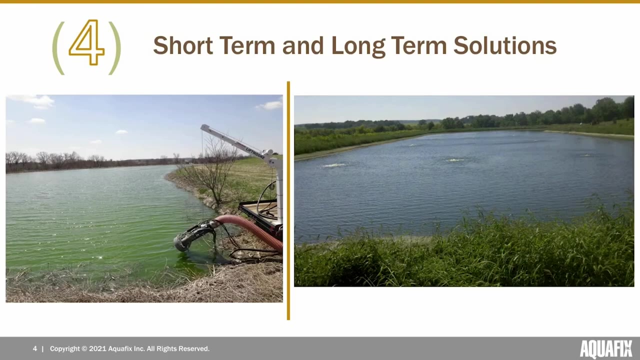 are harmful algae blooms. Second, we're going to compare and contrast harmful algae to green algae. Third, we're going to take a look at the environmental conditions that support the growth of HABs within a wastewater lagoon. This is all going to lead to our solutions, both in the short 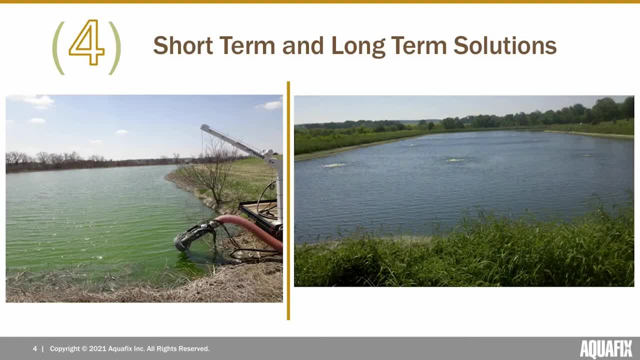 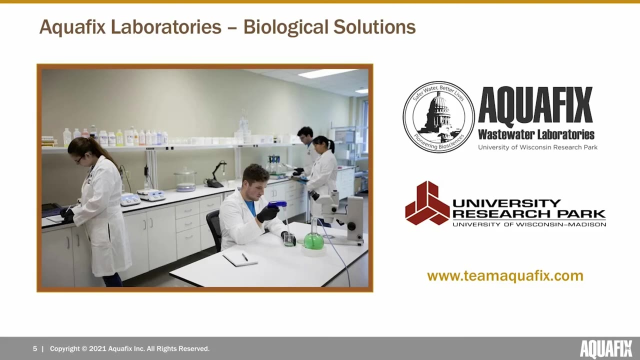 term and the long term for effectively treating and limiting the growth of harmful algae within lagoons, so that your lagoon can look healthy, nice and not completely green like we're seeing on the left hand side here. So our work, sample analysis and research at Aquafix is all being 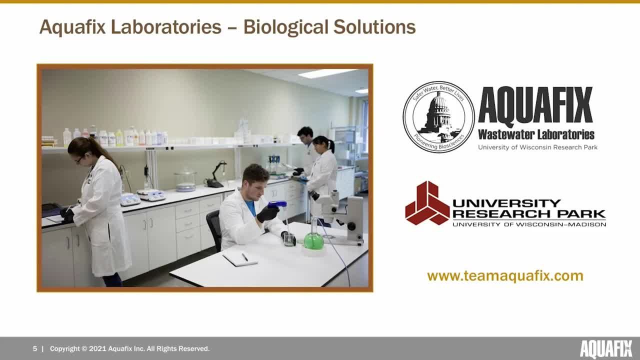 conducted in our lab at Aquafix, We're going to take a look at the environmental conditions that support the growth of HABs within a wastewater lagoon And we're going to take a look at the questions from those as we try to ameliorate our works with the L Eldridge Museum's. 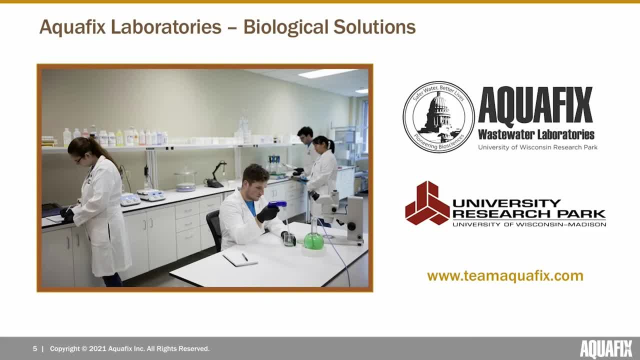 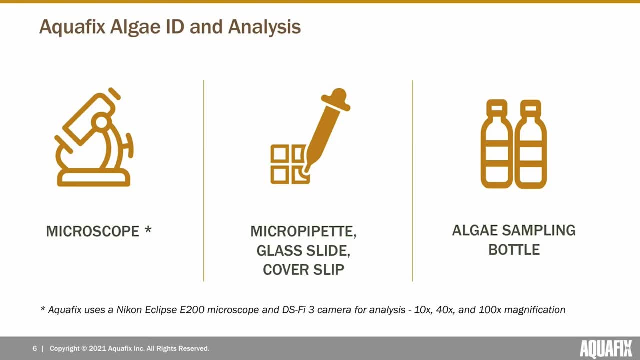 component of our ci-tion specialization project, plus some of our research labs at the University Research Park in Madison, Wisconsin. Our research labs here are the foundation for our treatment solutions, as well as our lagoon and algae research. Our research labs are also the 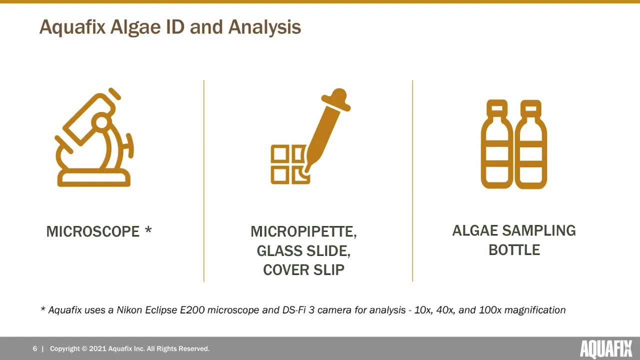 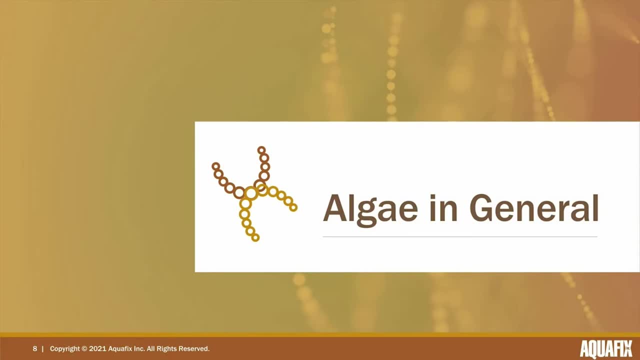 foundation for our algal ID and analysis, where we can provide algae ID and information for an algae sample that we see from a wastewater treatment system webinar. I would first like to talk about algae in a broad sense. Algae are a diverse group of 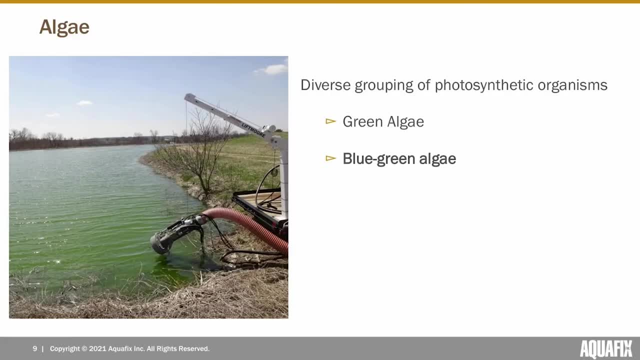 photosynthetic organisms, Algae are going to be larger than your typical heterotrophic bacteria that really act as the base of wastewater treatment, but, for the most part, are still going to be on the microscopic scale when it comes to actual identification. For today's webinar. 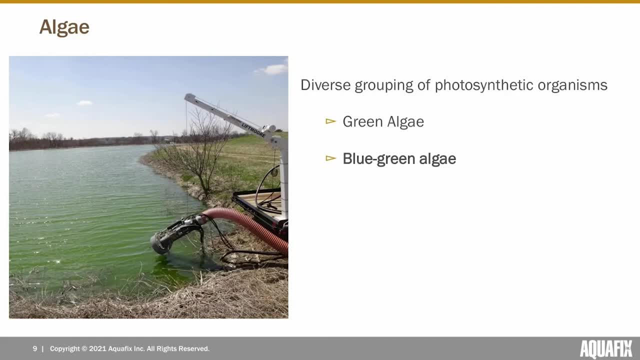 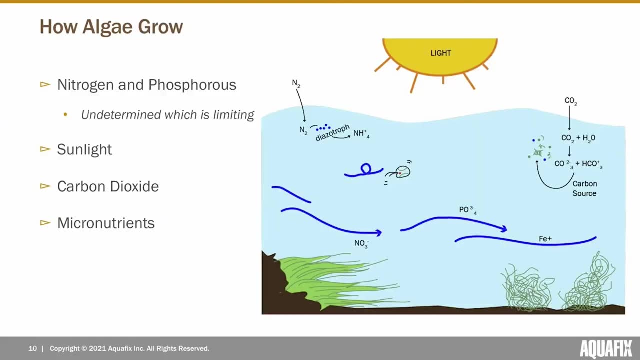 algae can be divided into two major groupings: your traditional and typical green algae, and then your blue-green algae or cyanobacteria. The basis for algal growth comes from sunlight and soluble inorganic nutrients such as phosphorus and nitrogen. Algae are also going to require 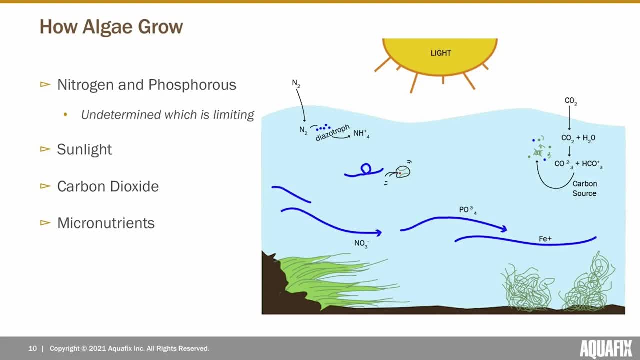 sunlight in order to photosynthesize and produce glucose. This process also mostly requires inorganic carbon- typically that's going to be CO2, to act as a carbon source for algae during the photosynthetic process. Regarding nutrients, nitrogen is often taken up as ammonium or nitrate. 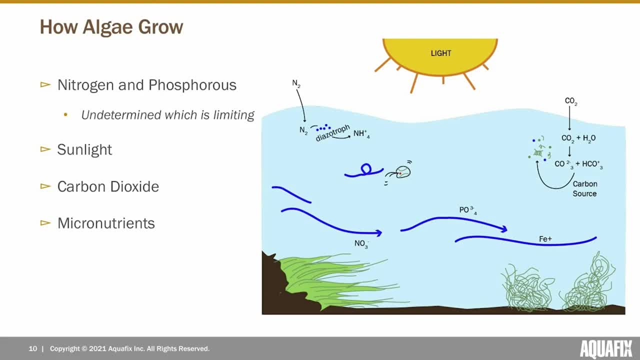 ion. However, in some cases, some cyanobacterial cells can fix atmospheric nitrogen and convert it into usable forms. Most algae take up phosphate from the water column as their source for phosphorus. It really is debated currently in the scientific community which nutrient- nitrogen or phosphorus. 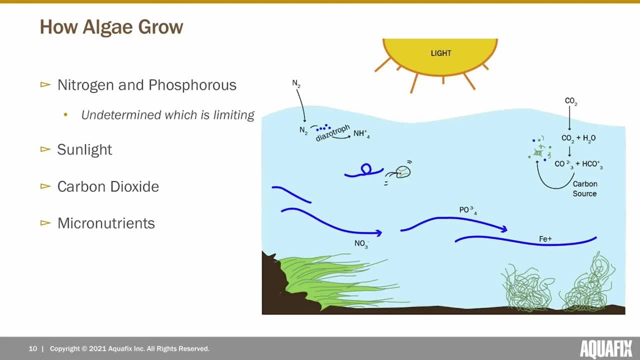 is going to be your limiting nutrient for the growth of cyanobacteria. One theory out there right now is that phosphorus is the actual limiting nutrient, as many cyanobacteria or nitrate ions are present within the water column, but in the case of algae it's going to be. 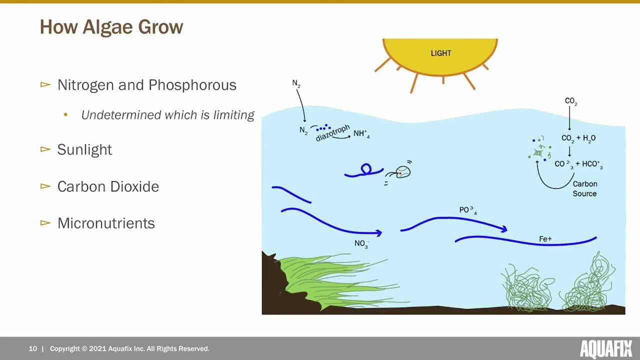 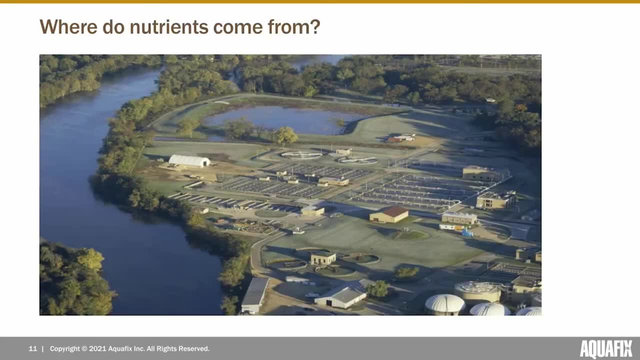 much more likely to be the case that phosphorus is going to be your limiting nutrient. Of course, various micronutrients are also going to be necessary to facilitate algal growth within a water body. So when discussing where nutrients are coming from, it's not going to be as complex. 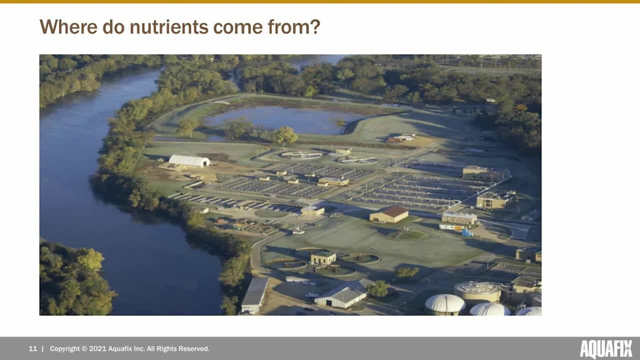 as discussing runoff or possible sources of pollution for a lake or river as wastewater. lagoons have a pretty direct point source of relatively high nutrient water incoming from a to the lagoon from the upstream treatment zones within your treatment plant. As this water will, 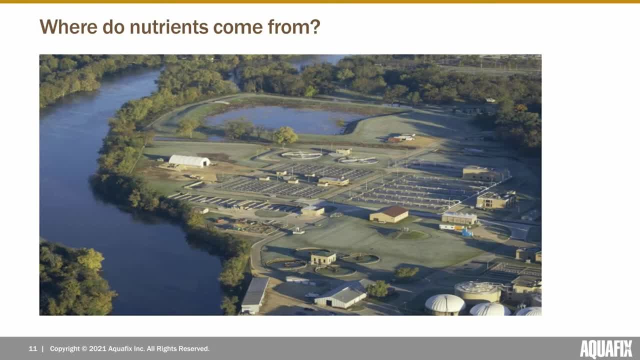 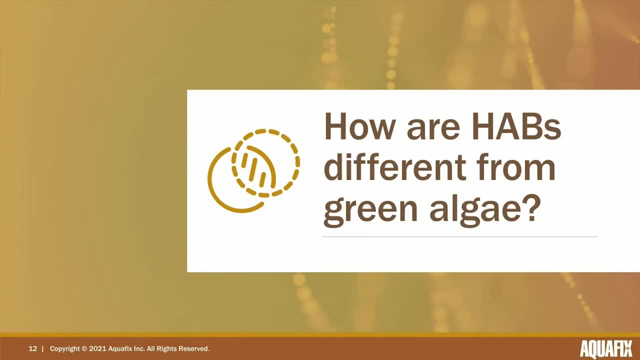 naturally have elevated levels of nutrients. this can make algal growth within lagoons all the more favorable, And so, when discussing algae growth within lagoons, it's going to be vital to discuss both the similarities and the differences in regard to green algae and cyanobacteria One. 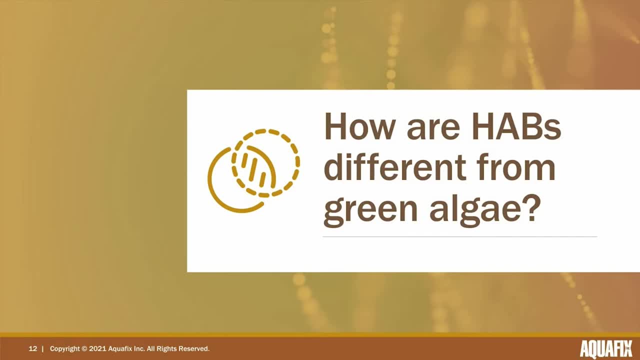 note is that when we're talking about harmful algae blooms and cyanobacteria, we can refer to them as those two terms as well as blue-green algae. These terms are all going to be synonymous for today's presentation, and you may see me switching back and forth between all of these. 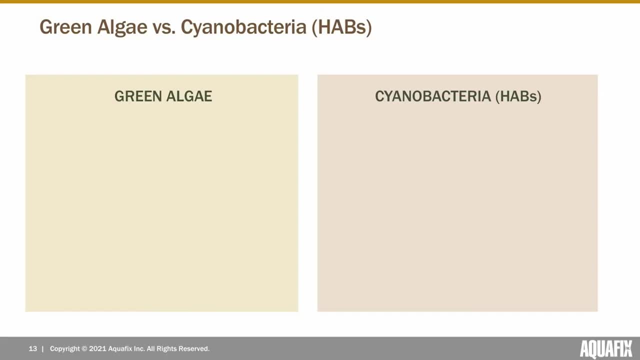 So we can start with some general similarities, as both these organism groupings are photosynthetic algae and have an innate ability to form surface blooms in wastewater, lagoons and other water bodies. Overall, these groupings of organisms are extremely similar, in regard to appearance as well. 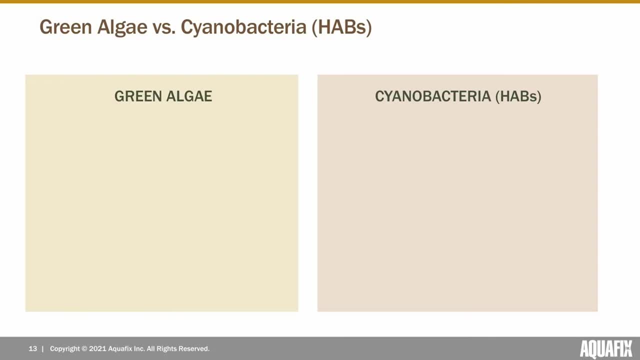 as environmental and ecological niche Within an ecosystem such as a wastewater lagoon. But now we can discuss what's important, and that's going to be the differences between these two groupings of organisms. Cyanobacteria are prokaryotic and from bacterial lineage, whereas green algae are eukaryotic and 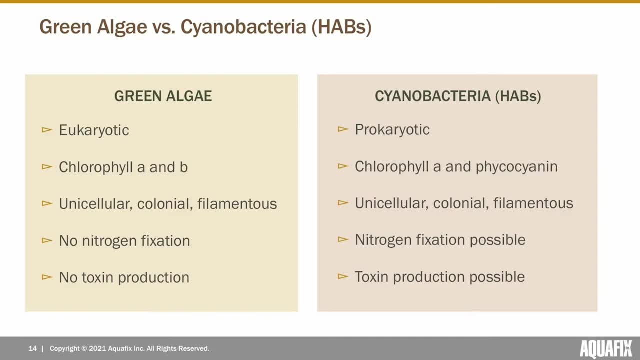 contain membrane-bound organelles within their cellular structure and more closely related to aquatic plants. However, both green algae and cyanobacteria are still able to conduct photosynthesis, although the pigments used to conduct photosynthesis are slightly different, And this is where we get this green versus blue-green coloration that can. 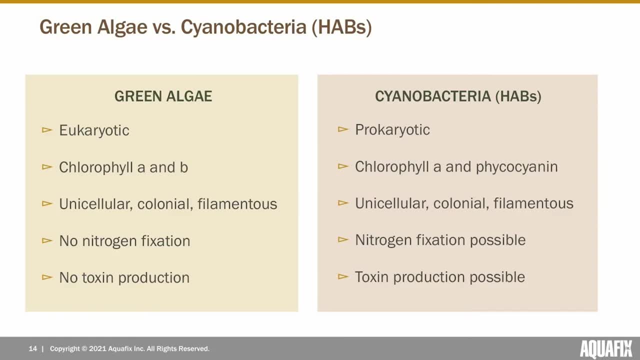 be observed between the two groupings. This is due to cyanobacteria's use of the phycocyanin pigment. Both green algae and cyanobacteria can have multiple forms, such as unicellular, colonial and filamentous. This is really going to depend on which species we're talking about within each. 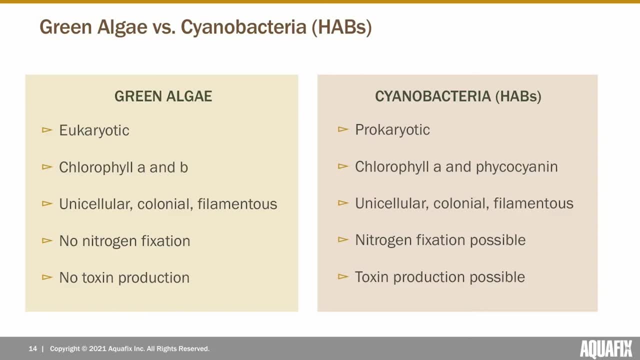 respective grouping. Finally, two other differences are going to be the ability of cyanobacteria to mix nitrogen from the environment, as well as the ability of cyanobacteria to produce toxins as a byproduct, And this toxin production has become a global issue in recent history. We're going to 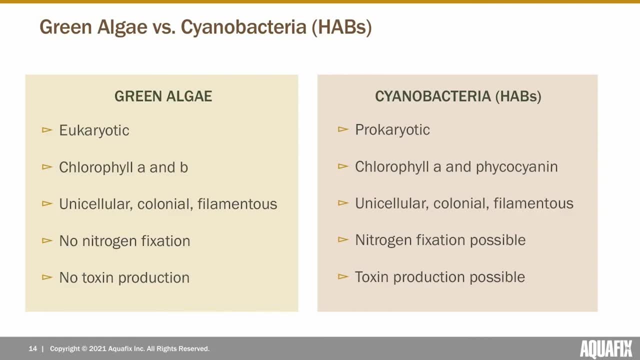 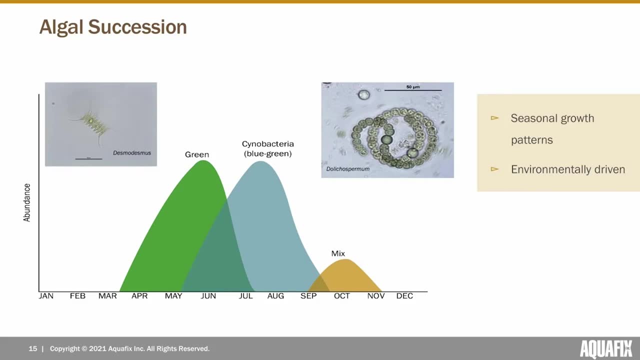 take a closer look at toxin production specifically later in today's presentation. The growth patterns of these two organism groups can also be different and seasonal, due to preferring different temperatures and the competitive balance that is found at these temperature ranges, For example, in spring, when 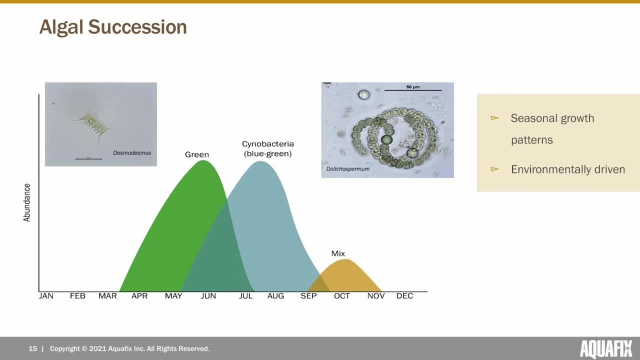 temperatures are high, cyanobacteria can produce toxins as a byproduct and this toxin production can are cool and just starting to warm up. We're going to see typically more nutrients within the water and we're going to see green algae being able to dominate at these slightly cooler temperatures. 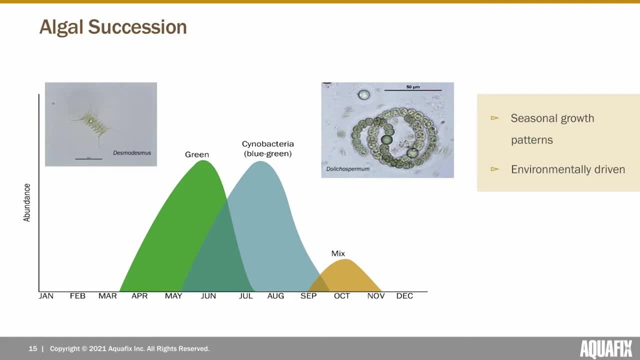 and make up the most of your algae populations. As the seasons progress to summer and we get higher temperatures, we tend to see more cyanobacteria being able to out-compete green algae and take over as the majority of algal cells within a water body In the fall as temperatures end up. 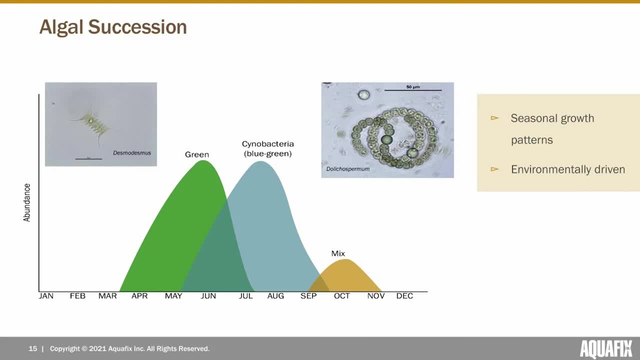 decreasing again, we tend to see more cyanobacteria being able to out-compete green algae and take over as the majority of algal cells within a water body. In the fall, as temperatures end up decreasing again, we tend to typically see a mixture between cyanobacteria, green algae and diatoms making. 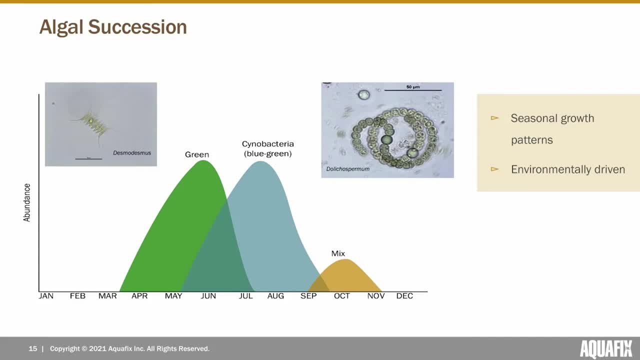 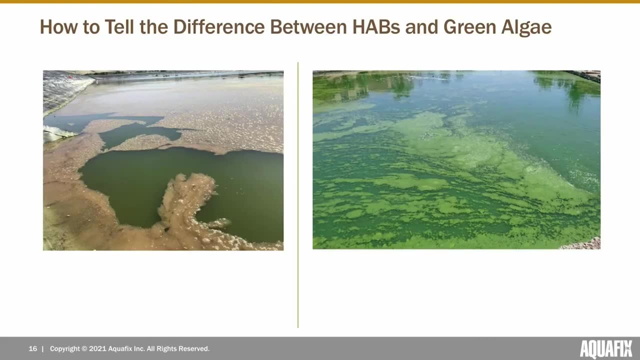 up your algal population as a whole. So these patterns are really going to be entirely environmentally driven, and that's what we can term the algal succession. So now I'd like to bring up the hypothetical question of it's summer. temperatures are hot, you begin to see a lagoon. 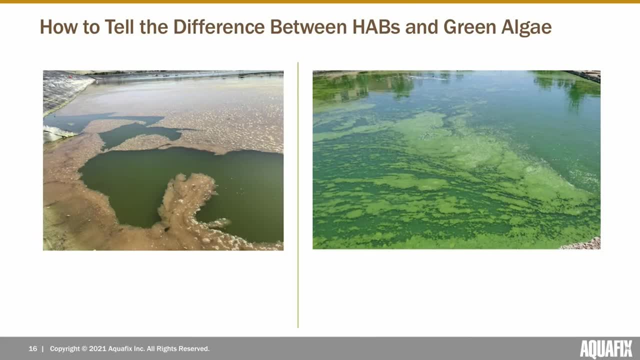 to start to turn green and a bloom of algae begins to form. How can we tell the difference from shore whether we are dealing with a green algae or a potential green algae? So we're going to toxic bloom of cyanobacteria. Unfortunately, there really is no simple answer to this question. 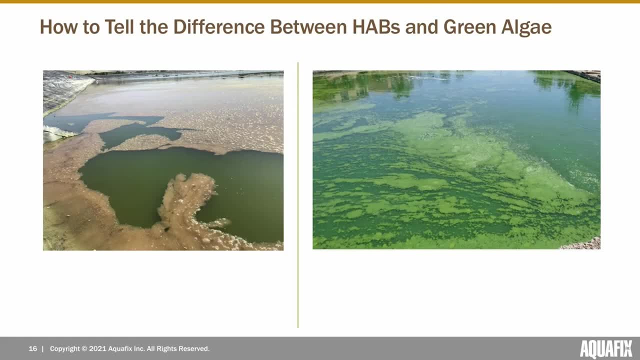 Here on this page we have two lagoons experiencing algae blooms, but from shore they're really both going to still just appear to be green water. Cyanobacterial blooms are often described visually as green pea soup or blue-green bright paint with streaks, but appearances can. 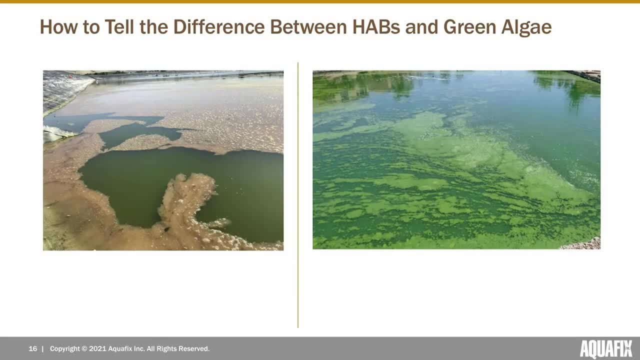 really vary based on what cyanobacteria is there and based on environmental conditions. Because of this, although you can give your best guess from the shore as to what you're dealing with, the only definitive way to know for sure what you are dealing with within your lagoon is going to be: 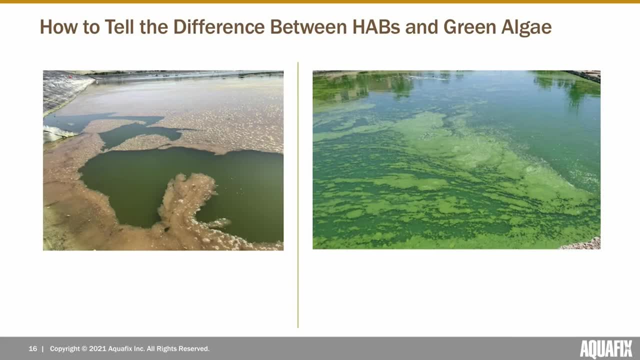 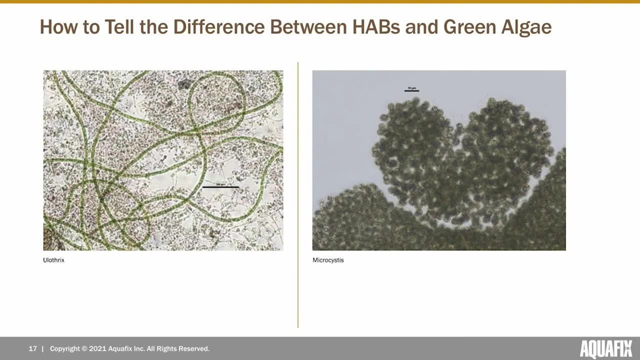 through microscopic analysis and algal ID. When looking underneath the microscope, it's going to be much easier to identify specific types of algae and make a correct determination whether you have a green algae or cyanobacteria On the left. when we look under the microscope, we see we found 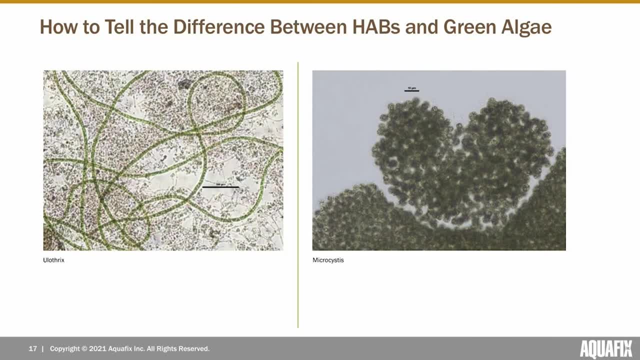 Ulithryx, which is a filamentous green algae. Mixed bacterial solids here, whereas on the right we have Microcystis, which is a unicellular cyanobacteria that is able to form colonies and can potentially produce toxins. A link should now. 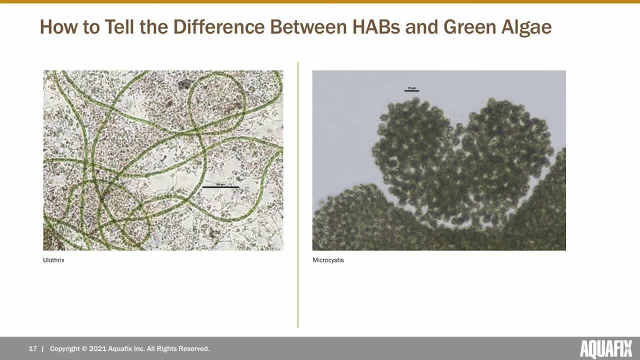 start to be popping up onto your screen and this link can take you to our wastewater microorganism database that we have, and this database is going to include images and descriptions of common algae and cyanobacteria that are found in wastewater treatment systems and lagoons. 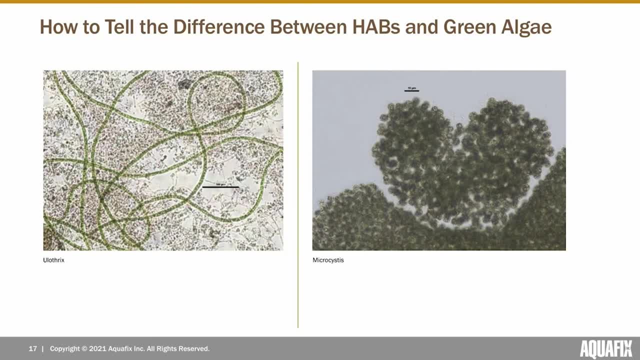 This database could be a good tool and use key for looking underneath the microscope and seeing if the algae that is being present within your lagoon is going to be a typical green algae or a cyanobacteria, And so that's a good use for everyone to use when trying to figure out what's. 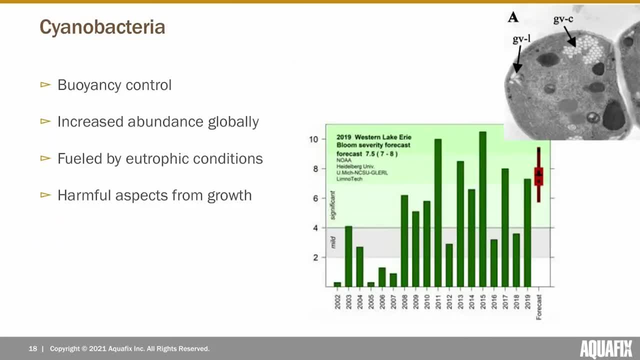 actually in my pond or lagoon, And so, moving on now, I'd like to discuss cyanobacteria specifically. There are some traits that make cyanobacteria a special concern for water resource managers around the world. The first trait is going to be buoyancy control, As many cyanobacteria are able to control. 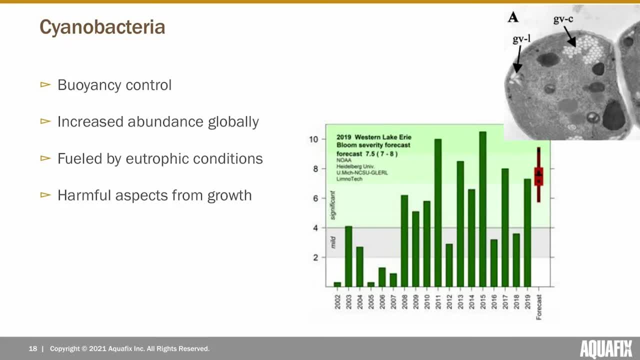 their vertical buoyancy through the formation of gas vesicles. As you can see in the top photo of a cross-section of Microcystis cell, the arrows there are pointing at gas vesicles. These gas vesicles allow HABs to regulate their buoyancy, to not only optimize environmental conditions. 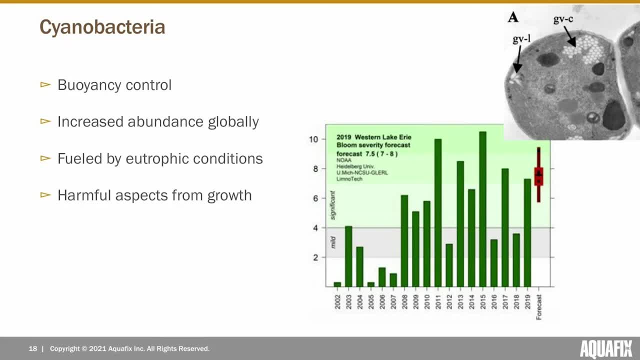 around them, but also rapidly rise to the surface and maintain surface blooms under optimal growing condition. Secondly, the presence of cyanobacteria is going to be a key factor in the development of cyanobacteria. This is going to primarily be fueled by these eutrophic conditions, or what can be. 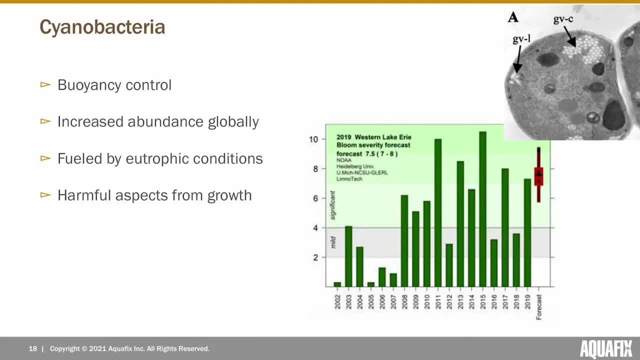 nutrient saturation of an environment, which is really unfortunately going to coincide with many wastewater lagoons. Next, there's going to be many harmful aspects of growth, such as toxicity, And, as I said, we're going to be covering the toxicity specifically later. Finally, HAB occurrences have 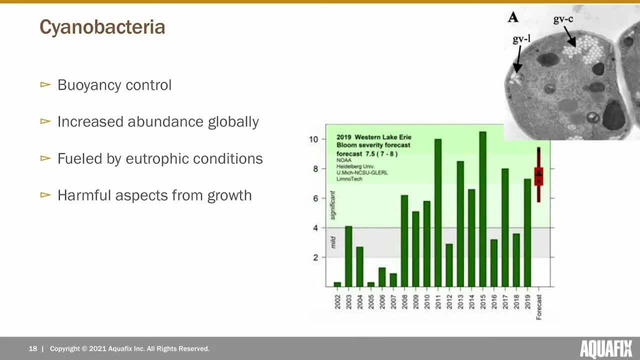 increased globally. As you can see from this chart, on the page of blooms found in Western Lake Erie, there is a pattern of increased HAB abundance, and this pattern of increased HAB abundance is only theorized to increase in the future as water bodies become more eutrophic and temperatures continue to rise, As we're expecting more HABs. 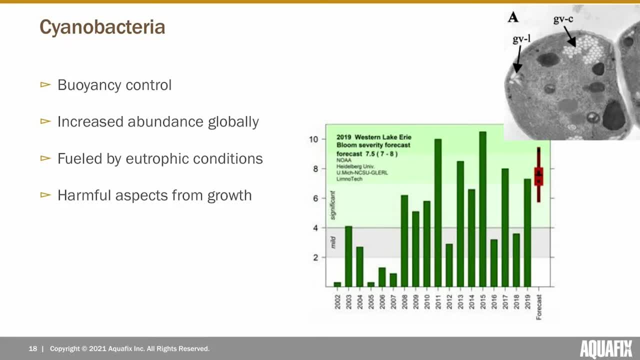 to be present in the future. this is why it's going to be incredibly important for wastewater operators and water resource managers to be prepared for an increase in abundance of HABs rather than being reactive to seeing more HABs within your lagoon. As I stated, HABs have 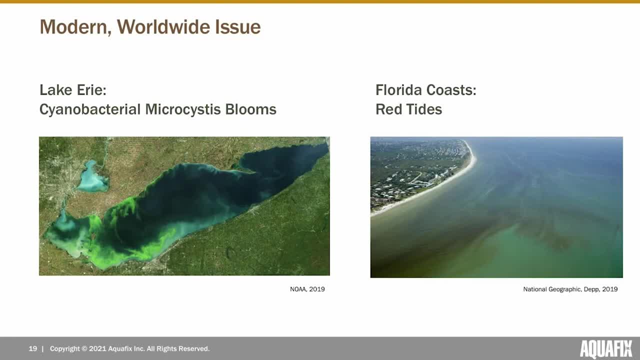 increased globally and they now become a modern, worldwide issue that the public does have a lot more information about. So, as I stated, HABs have increased globally and they now become a modern, worldwide issue that the public does have a lot more information and knowledge on. We have two. 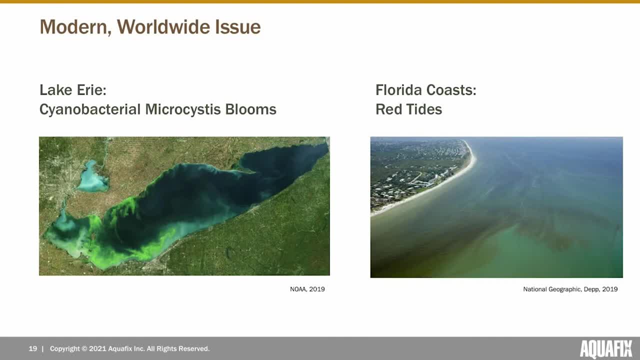 different types of HABs shown here. We have microcystis blooms in Western Lake Erie that have at times troubled the water supply of many Ohio cities due to the presence of cyanotoxins. We also have a dinoflagellate-driven harmful algae bloom on the coast of Florida that can cause seafood. 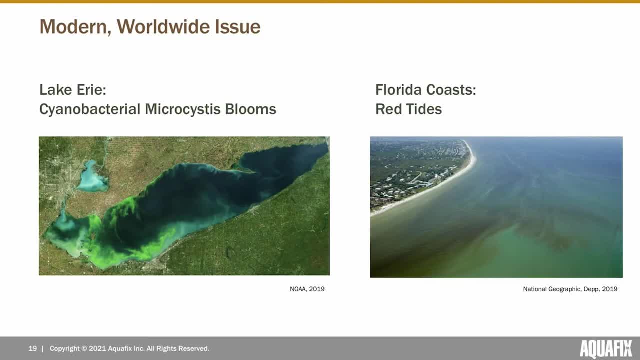 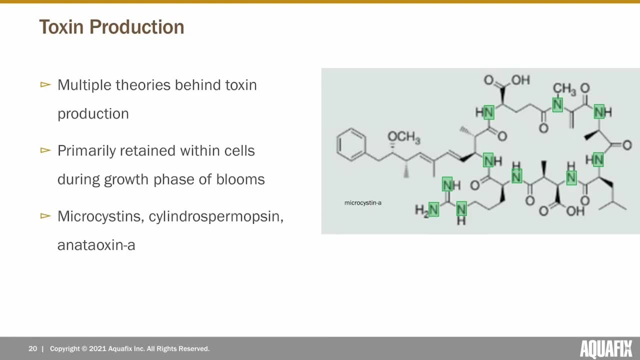 toxicity in dangerous waters for recreation. So it really is a modern, worldwide issue that's going on today And so, as I stated, we were going to talk about toxicity a little bit more in depth, and when we're talking about toxicity, we're going to talk about toxicity in depth, and when we're 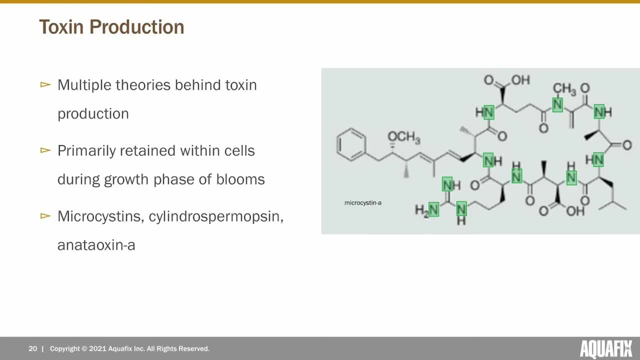 talking about toxicity, it's interesting to pose the question of why are these tiny, microscopic organisms releasing toxins in the first place? As you can see from the microcystin, A toxin molecule on the page, the production of microcystins by microcystis is going to be a really an 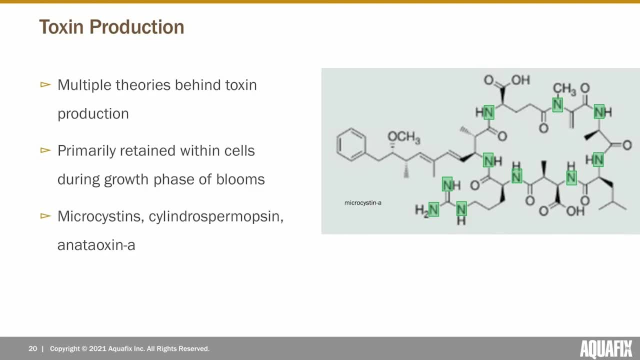 energetically intensive process that requires a ton of nitrogen. So the molecule we're looking at is just a single toxin molecule produced by cyanobacteria, and there's a ton of nitrogen packed in there. Because of that, it really makes you think about the fact that there's a lot of 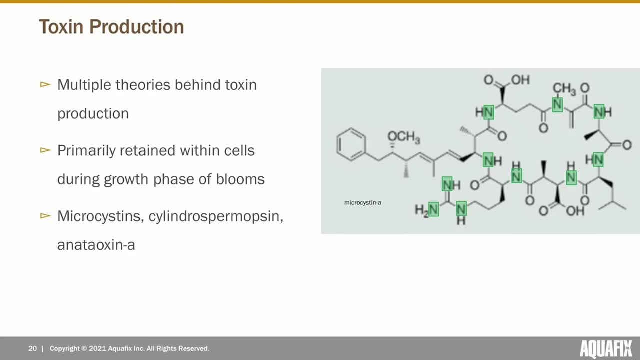 toxin production. And so we're going to talk about the toxicity of microcystin, A toxin molecule, by the way, and then we'll talk about the toxicity of microcystin, A toxin molecule. Unfortunately, there is no clear consensus right now for the reasoning behind toxin production. 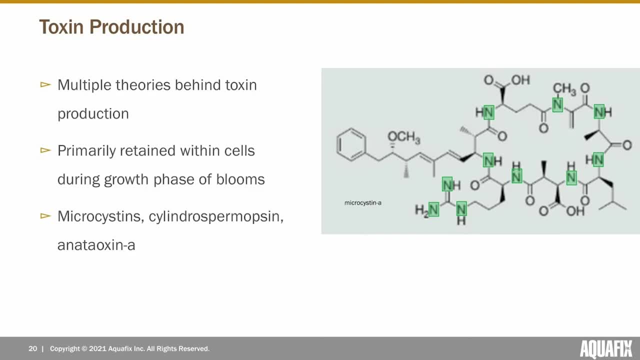 but there are many theories for why toxin production could provide HABs an evolutionary advantage over your green algae and other organisms. One of those options is self-defense. This could be self-defense against possible predation and other organisms. Another option is that there's just some unknown reason that we aren't sure of, And I kind of fall into that. 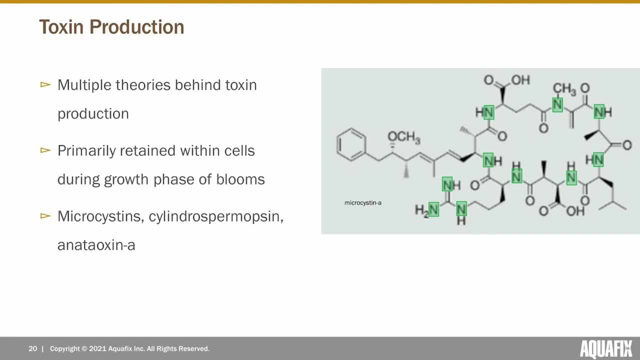 place that we just don't know why these cyanobacteria are releasing these mass amounts of toxins. Some toxin compounds can be referred to as microcystins, cylindrospermopsins, as well as anatoxin A. It's important to note that toxins are not always produced and the presence of 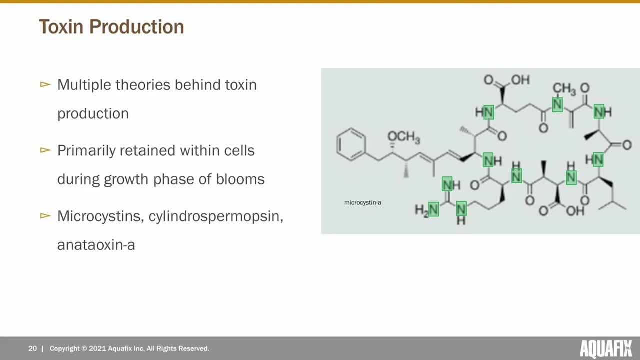 toxins is not always produced, So it's important to note that toxins are not always produced is not always going to be predictable, as well as toxins can be retained within harmful algae cells during bloom formation, whereas cell lysis is where we see a large expel of. 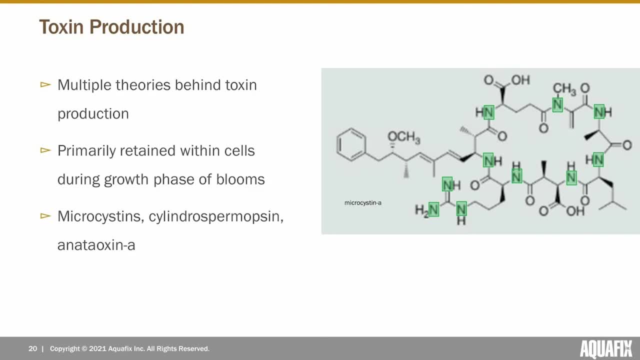 toxin concentration. In some cases, toxin production has been linked to higher levels of nitrogen present in order to support the formation of these toxin molecules, as you can see. So when we're talking about the toxins, we're talking about toxin release from lagoon. 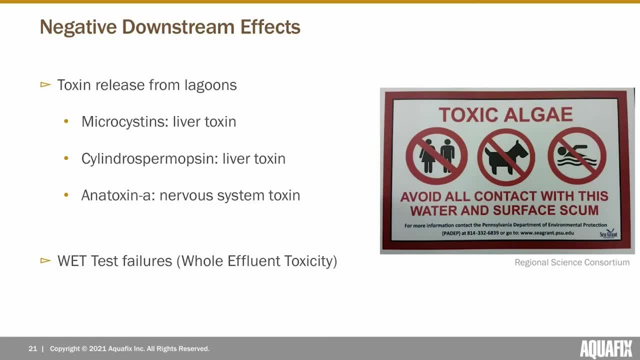 specifically, This can have many immediate as well as downstream effects, not only on the people that are managing the lagoons, but also the people that are downstream from the lagoons and affected by a lagoon's effluent discharge. These toxins, although relatively short-lived within the environment, can present. 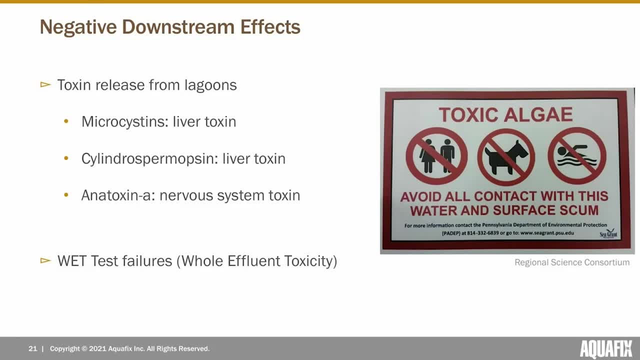 many dangerous side effects when coming in contact to people, animals and particularly- as I'm sure many of you have seen on the news, sadly- dogs. This can come through inhalation, contact and consumption within a water body that contains a high concentration of. 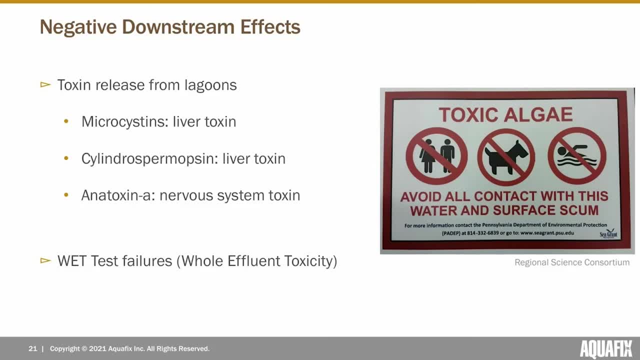 for example, cyanotoxins, Microcystins and cylindrospermopsin, can be produced by multiple different cyanobacteria and can be categorized as liver toxins, whereas anatoxin A is going to be a fast-acting toxin that affects the nervous system. Besides that, toxins affect 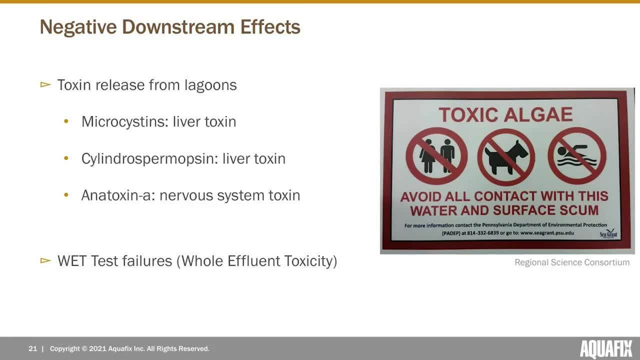 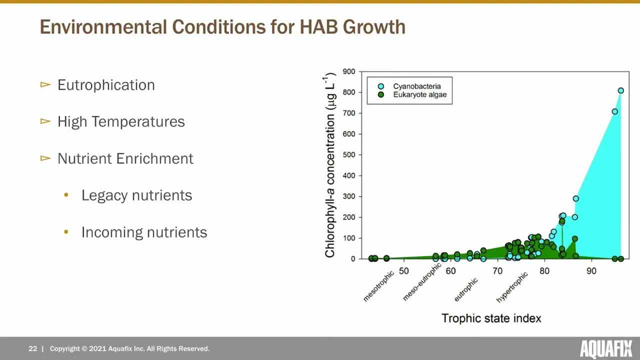 a human and animal life failure of your plant's whole effluent toxicity testing could also be risked if cyanobacteria are present and producing toxins. So within wastewater lagoons, the environmental conditions that are present can make for optimal growing conditions for not only algae but specifically cyanobacterial HABs. 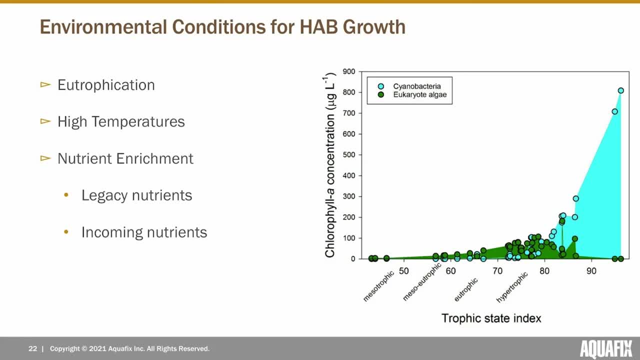 Due to the consistent nutrient enrichment of wastewater lagoons from both incoming nutrients from the upstream treatment process as well as legacy nutrients already present within the lagoon. this, combined with high temperatures and the trophic state of your water body, is going to likely lead to predictable formation of HAB blooms, As you can see in the graph. 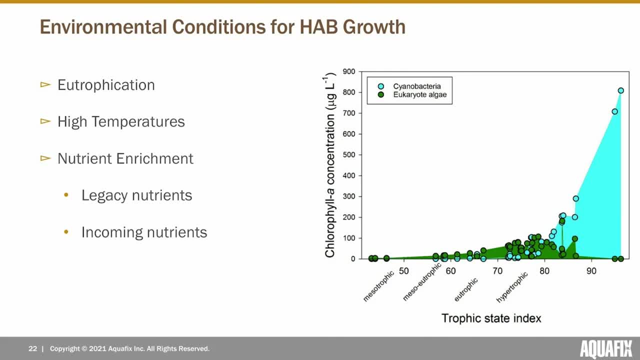 there is a shift in abundance from green algae to cyanobacteria, as the trophic state of a water water body or the amount of nutrients present within that water body are increased due to eutrophication and excessive nutrients, So as our focus has primarily remained on nutrient, 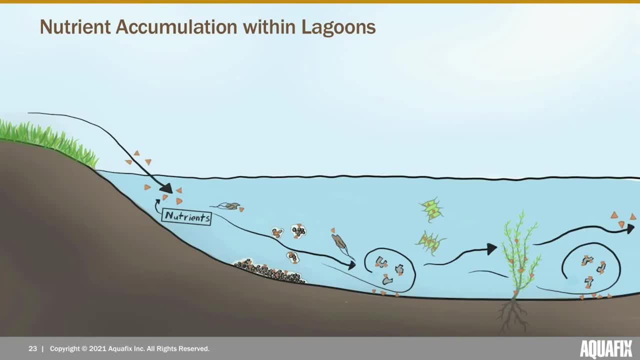 availability, leading to this spur of HAB growth. I'd like to take a moment to discuss the process of a nutrient accumulation within the water column and sludge of lagoon. Obviously, there is a point source: input of nutrients from the upstream treatment process that's going to 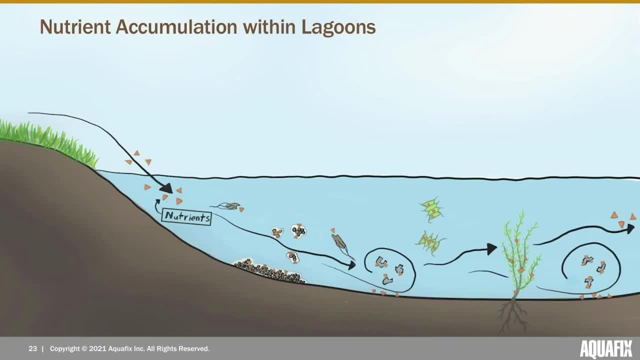 perpetually introduce nutrients within a wastewater lagoon, You're also going to get atmospheric nutrients. you're going to get runoff into the lagoon as well, as you're going to get sediment nutrients, contributing to the nutrient reservoir of the lagoon as a whole. The fate of 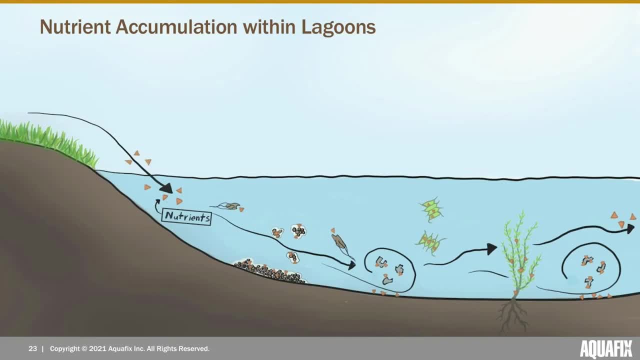 nutrients can have many outcomes, such as attaching to solids or absorbing to other chemical compounds within the water column or within the sediment layer. Nutrients can also be utilized by bacteria, by plants and algae, or just simply stay suspended on their own within the water column. As nutrients continue to accumulate within a water body, we can begin. 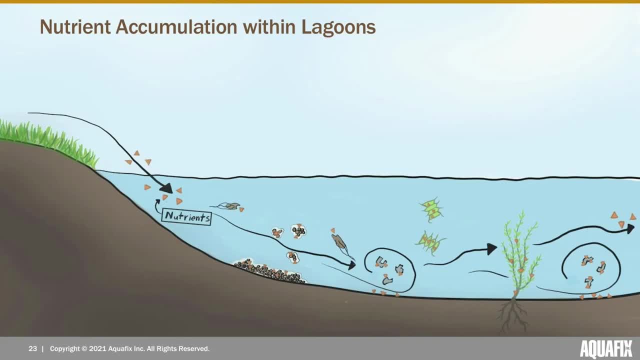 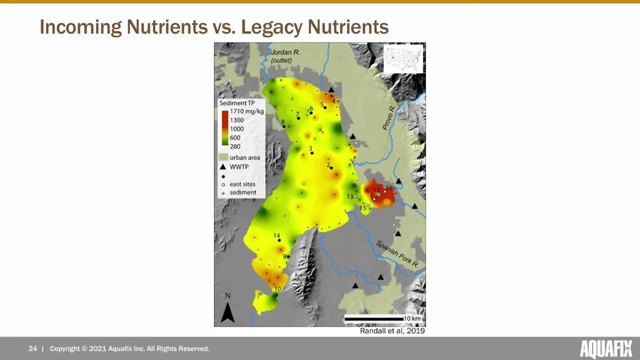 to see cyanobacteria and other algae being able to have a competitive advantage and eventually begin to form blooms within a water body. An example of this process of nutrient accumulation can be found in a recent study that was focused on sediment characteristics and HAB growth in Utah Lake. 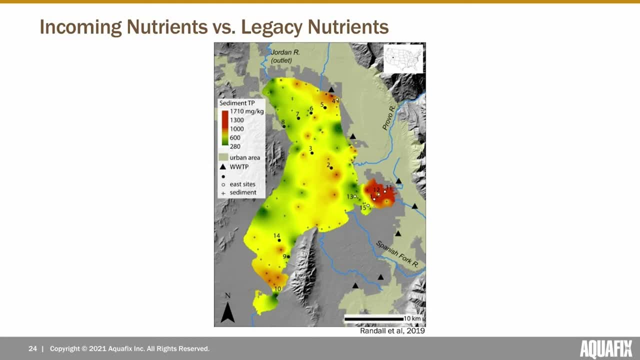 located just southwest of Salt Lake in Park City. Specifically, researchers here were analyzing the sediment, pore water and water column nutrients. These calculations include specific parameters of carbon concentration and commentaires on the downtown EPA' 根液 level and environment for nutrient accumulation levels in relation to where they were finding these common locations of repeatable HABs. As you can see from this map, phosphorus concentrations were primarily concentrated toward urban input areas, wastewater treatment plants, and bottleneck areas and coves. As you can see, the wastewater treatment plants are notated with triangles on the map, as well as the light beige color is notating your urban inputs. 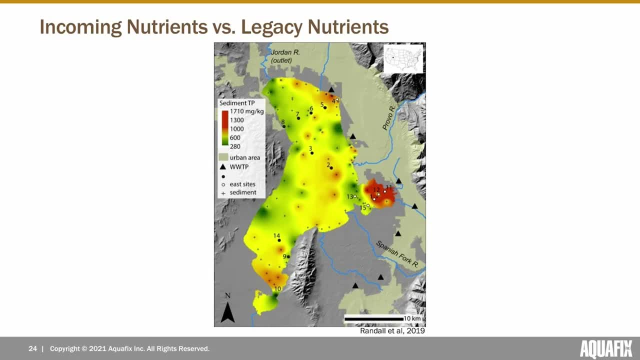 And so, as you can see from the map, your elevated levels of sediment and water concentration in the lake'sâmrid layer are important to help you determine the rate of reduction by the weight of the reserves. Water can't always be enough to move the waste to the consistent area of the water, but we certainly can compare that to the quality of the waste, which we did in this study. 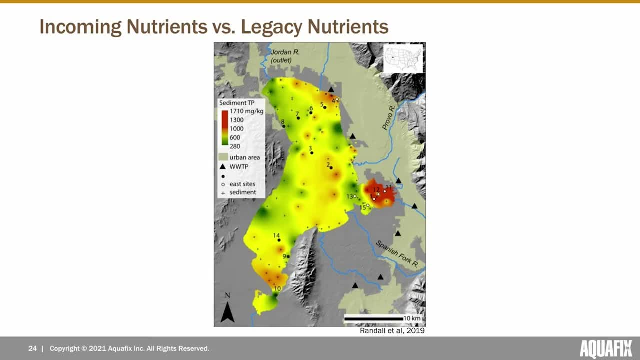 And so, as you can see from the map, your elevated levels of sediment and water column, phosphorus, were associated locally near these discharge sites from, rather that be, urban inputs or wastewater treatment plants. This study went on to find that HAB growth was also associated locally to these sites. 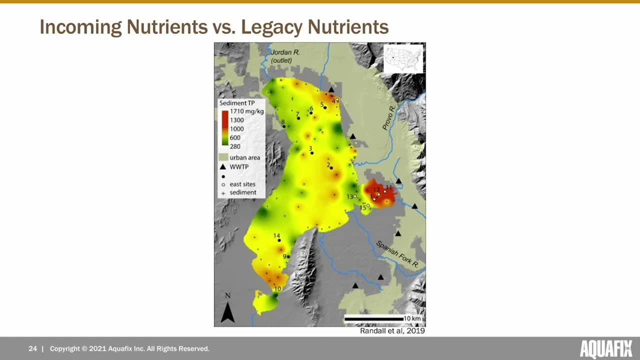 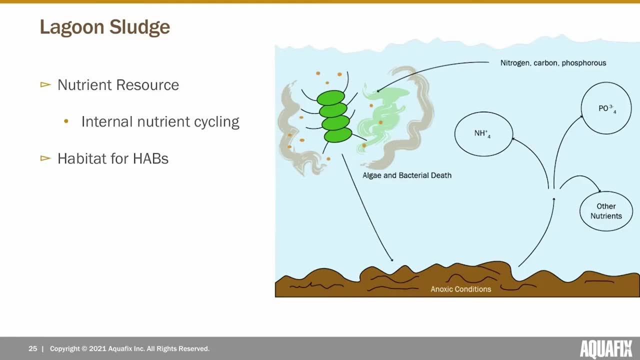 with higher levels of sediment and water, column, phosphorus- as well as locally near these urban inputs and wastewater treatment plant discharge sites. So when specifically looking at that sludge layer within a lagoon, it's important to remember that it's going to continually build up due to dead and decomposing bacteria algae plants. 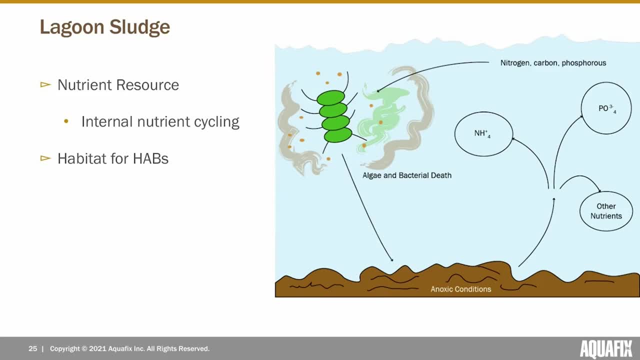 animals and other organic and inorganic solids within your lagoon. Heterotrophic bacteria can utilize this sludge as a food source by breaking down its organic matter. However, this nutrient dense sludge can also be responsible for fueling harmful algae blooms. 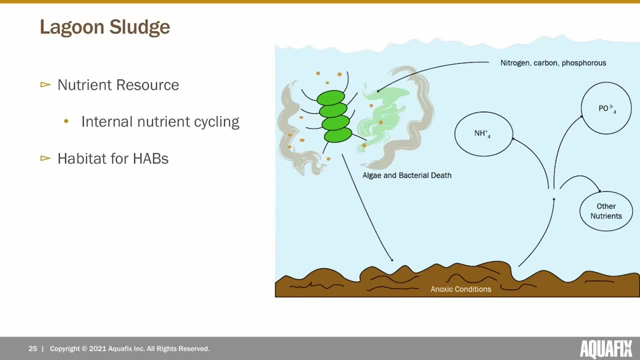 And this is true even when incoming nutrient levels are low from upstream treatment. This is because sludge sediments are able to hold nutrients such as nitrogen and phosphorus, and these nutrients can be released due to the physical resuspension of sediments. as 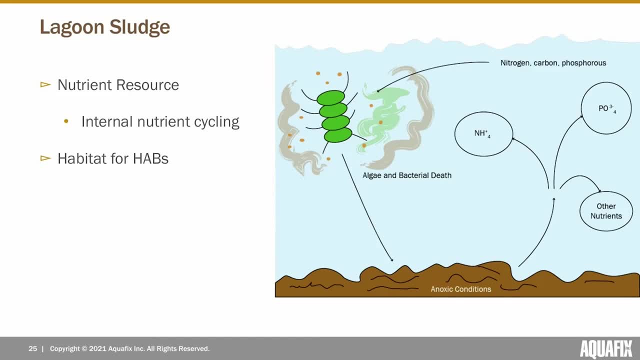 well as due to anoxic conditions leading to the release of internal nutrients from the sediment layer back into the water column. Higher sludge depth and sludge buildup can lead to more anoxic conditions and subsequently lead to nutrient release and, eventually, algal growth in the water column can be caused by. 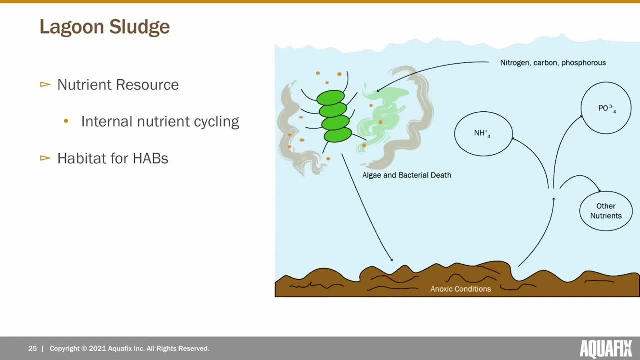 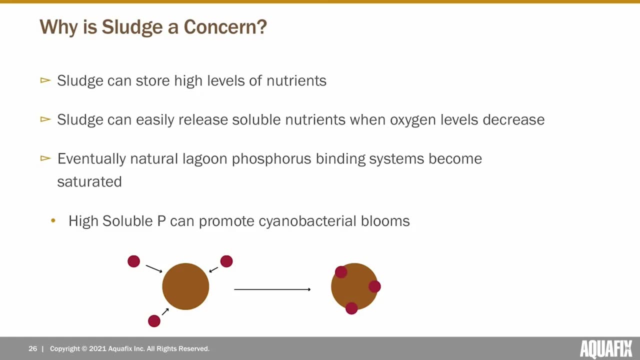 anoxic conditions. This can be especially true if there is a proportional lack of soluble carbon within the water column, And so, because of all, this excess sludge within a lagoon can be a major concern, And this is a major concern because it can be causing these repeatable HAB blooms and 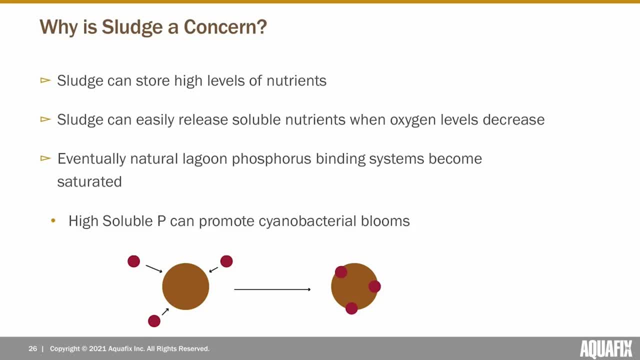 favoring this detrimental cycle of nutrient release from the sediments, an algal bloom and a subsequent algal crash and eventually the buildup of more sludge after that algal crash and cell death. This cycle is really primarily driven by a lagoon sludge's ability to store those nutrients as well as release those. 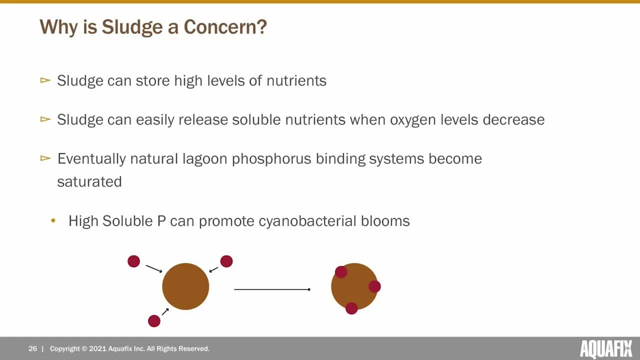 nutrients. under certain environmental conditions, such as anoxic conditions. Also, within lagoon sediments, phosphorus binding sites can eventually become saturated and this can lead to proportionally higher levels of phosphorus remaining within the water column rather than binding into the sediment layer. 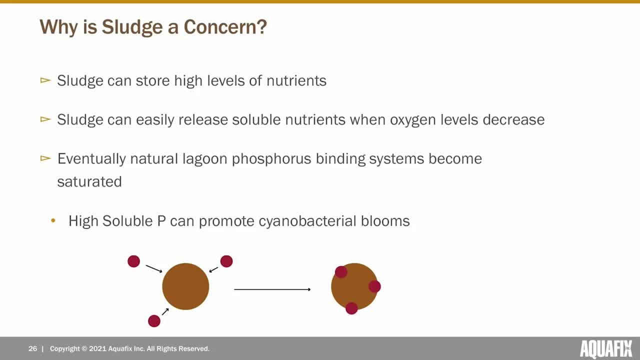 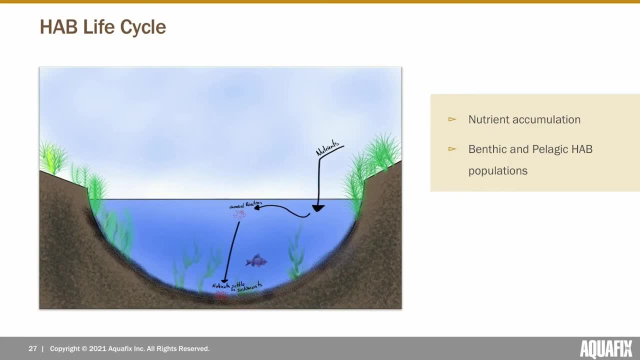 Higher levels of phosphorus within the water column proportionally can actually favor the growth of cyanobacteria over your standard green algae, And so I'd like to now show this repeatable cycle of cyanobacterial HAB blooms visually within a water body. 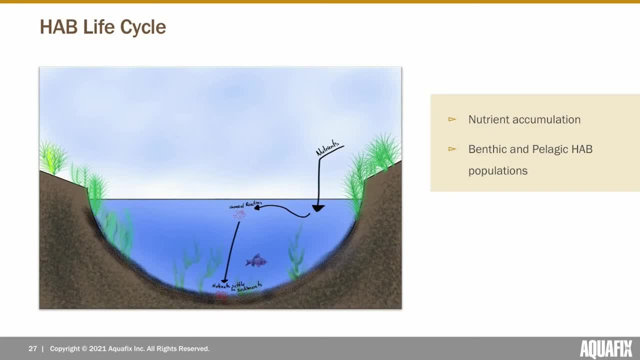 The beginning of the cycle starts with two populations of HABs. You have benthic or within the bottom sediment, and pelagic or within the water column. These separate populations can be present in low numbers and really not be causing any. 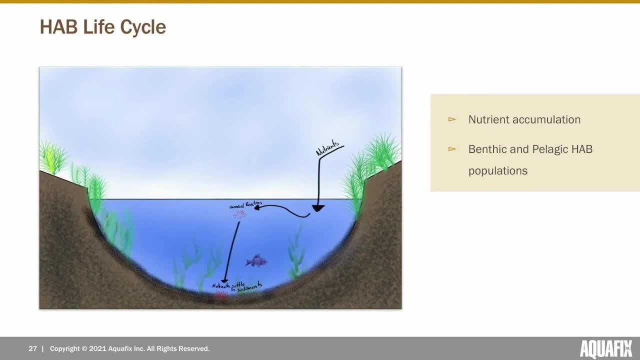 issues at all. However, over time, nutrients can begin to enter the pond and stay suspended within the water column or settle into the sediment layer, very similar to the HAB cells. As more and more nutrients enter into a lagoon system, the sediment can become eventually saturated. nutrients can be released. 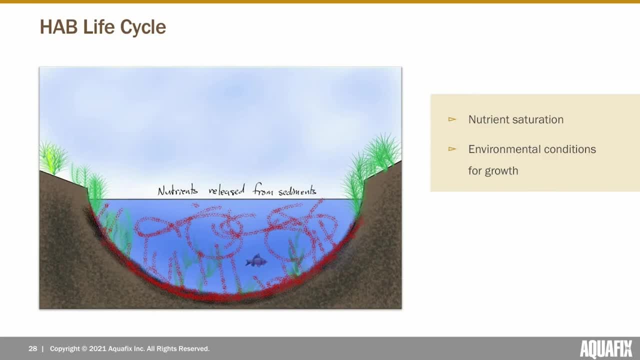 internally, as we discussed, and optimal growth conditions can begin to occur for those harmful algae cells. Due to the natural buoyancy control of HABs, both the sediment and pelagic populations are able to rise to the surface and begin this growth process. 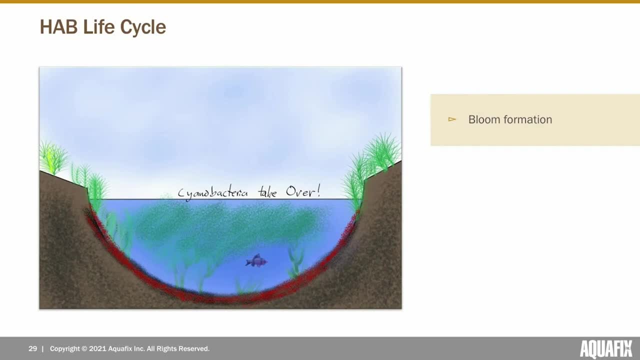 As you can see, now these harmful algae are really going to be able to take over, consume those excess nutrients, continue to direct their buoyancy upward towards light, and can rapidly take over a water body. Thank you, Have a great day. 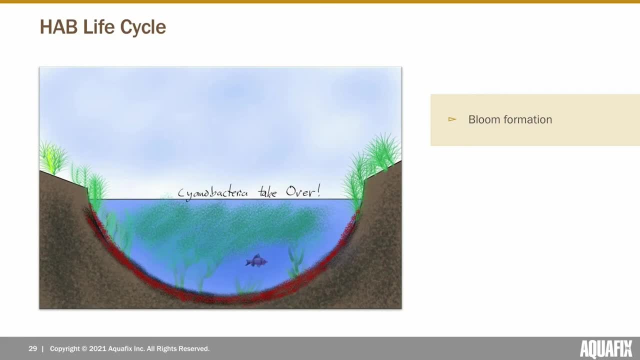 And we'll see you next time. Bye-bye, Bye-bye, Bye-bye, Bye-bye. This cycle of nutrient levels increasing- cyanobacteria will take over- can be habitual, And this is really going to be due to eutrophic conditions remaining present and the rapid 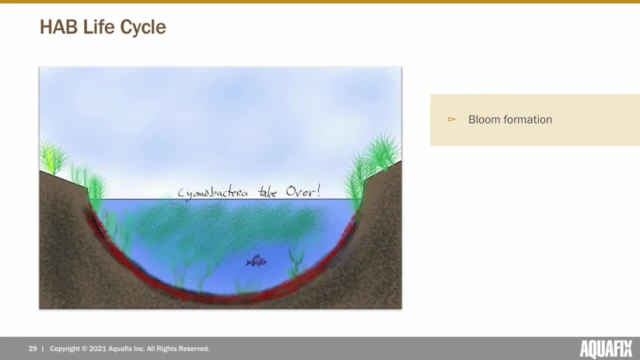 proliferation of cyanobacteria under optimal conditions. During the second half of this presentation, I want to discuss the effect that HABs can have on lagoon systems specifically, as well as some solutions that we can provide to help prevent and control the growth of HABs within a wastewater lake. 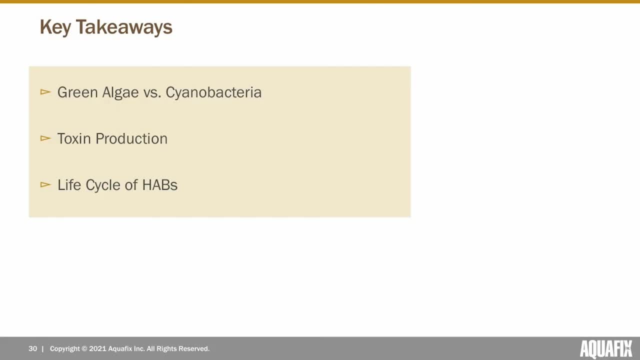 lagoon. But first I'd like to just give some takeaways before moving on. I want to reiterate that it's important to remember that green algae and cyanobacteria, although they are very, very similar in the fact that they are photosynthetic organisms that can appear green on the surface of 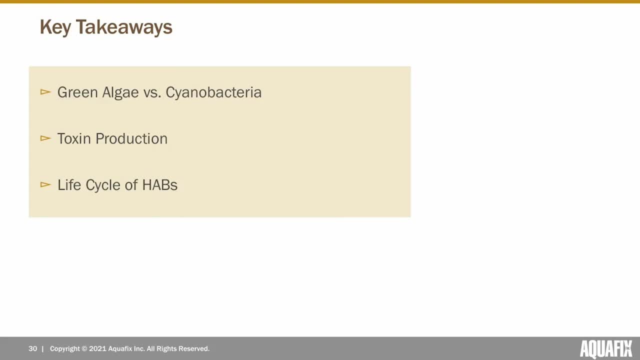 your water body. they are very different still, And one of those largest differences is the ability for cyanobacteria to easily produce toxins within your water body, And I also want to then reiterate that life cycle of HABs that we continually see being fueled by eutrophic. 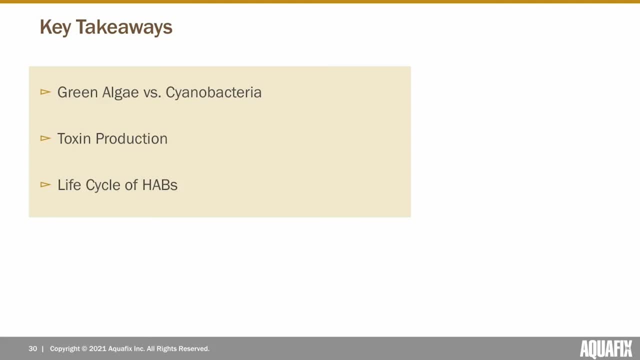 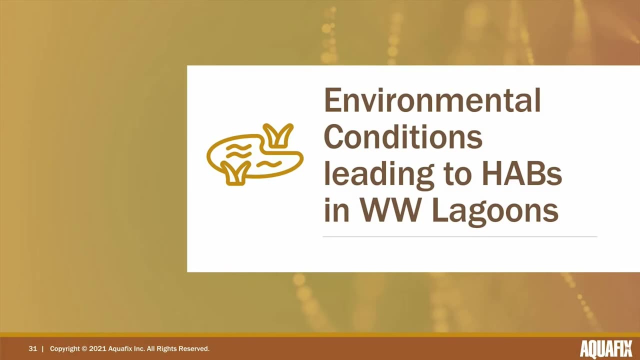 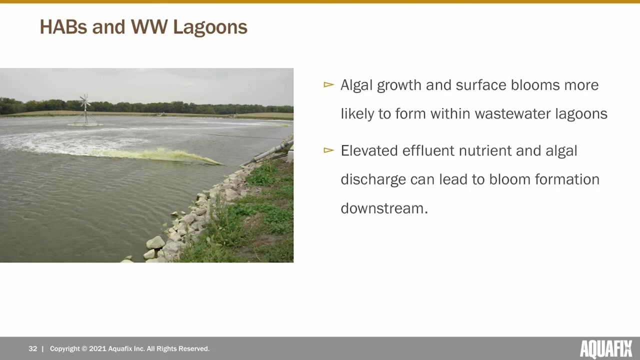 conditions and eventually being able to take over a water body. And so as we begin to move on and talk a little bit more specifically about wastewater lagoons and the conditions within lagoons that can lead to HABs, moving on to the next, really second half of this presentation, 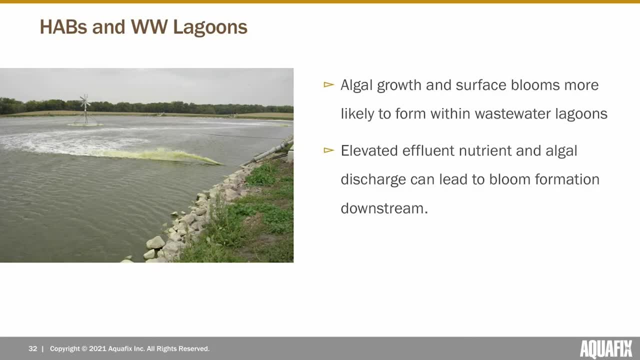 I'd like to discuss HABs in reference to wastewater lagoons specifically as our primary growing system, As we discussed earlier. in many ways, wastewater lagoons provide the perfect environment to support the growth of algae and harmful algae. Because of this, an opportunistic cyanobacteria can swiftly 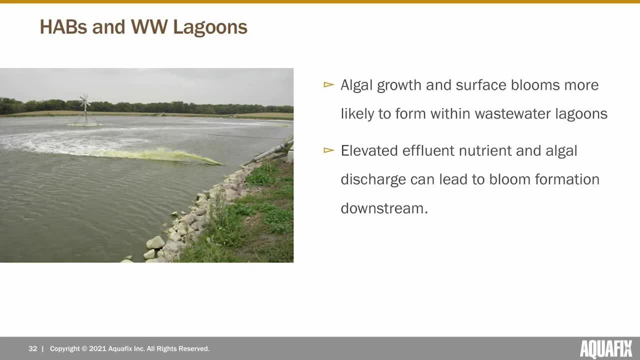 explode in abundance and we can see bloom formation occur Outside of the lagoon. we can also have negative downstream effects in public waterways from both elevated nutrient discharge and elevated algal discharge from a wastewater lagoon after a bloom has developed, And this can 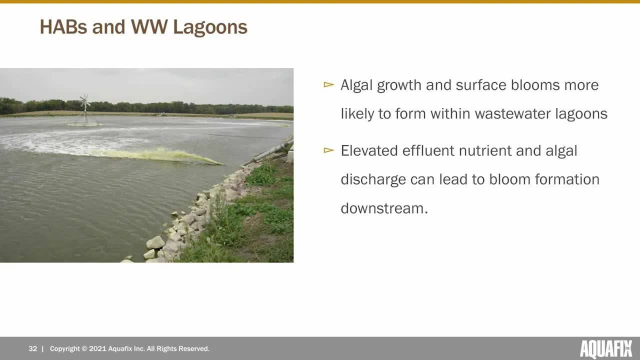 eventually lead to a loss of algae And so, as we've discussed earlier, in many ways wastewater lagoons can lead to this HAB bloom formation. downstream HAB prevalence is not only going to be a wastewater lagoon issue, but can also really be a community issue downstream from a wastewater. 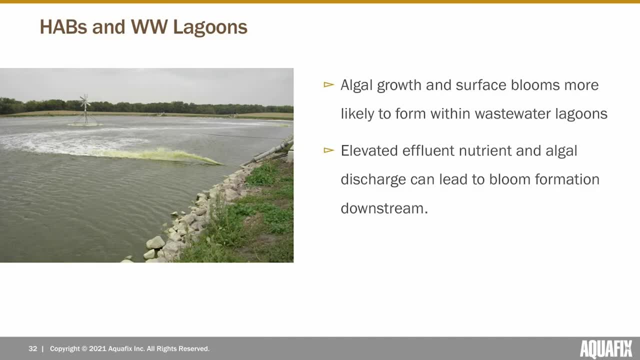 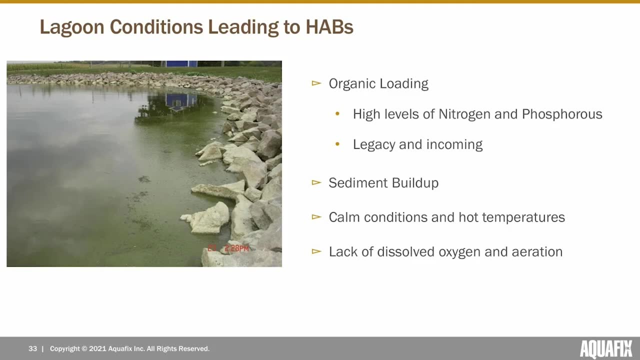 lagoon due to the flow of algal cells, nutrients and toxins. So looking closer now at the specific lagoon conditions that can lead to HABs, we can start with the excessive amount of point source: organic loading coming into a wastewater lagoon from the upstream treatment process. elevated levels. 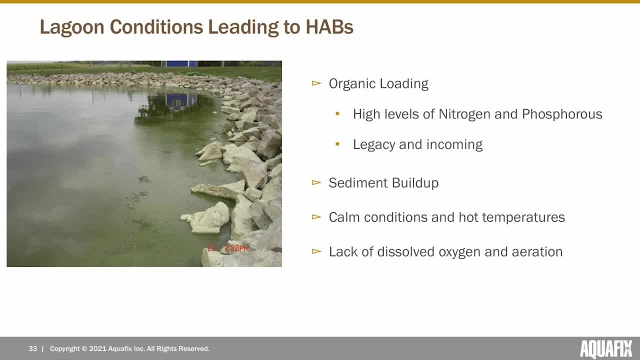 of nitrogen, phosphorus and organic solids will flow directly into a lagoon And even with effective treatment upstream, in almost all cases this type of nutrient and solids loading will outweigh the typical lake or pond. And besides the incoming nutrients from upstream, we also see that 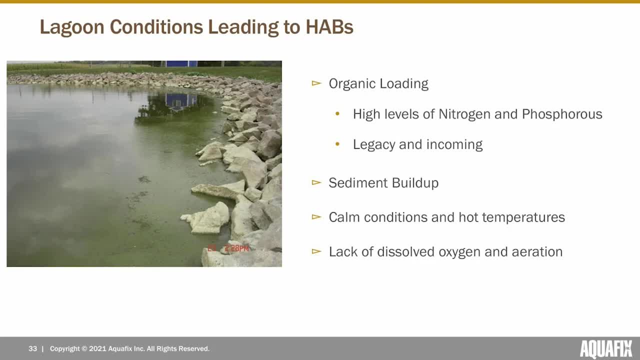 the legacy nutrients within the lagoon that are internally cycled can also contribute to those conditions. Internal nutrient buildup can lead to those predictable blooms. as I had stated, due to the addition of nutrients, Legacy nutrients are going to be largely retained within the organic. 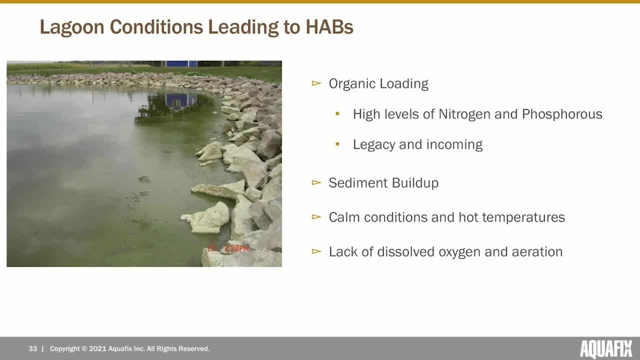 sediments on the bottom of your wastewater lagoon, And as sediment builds up over time, it can hold more nutrients as well as act as a larger habitat for HAB cells and resting structures. Finally, in combination with that sediment buildup, calm conditions, hot temperatures and a lack of 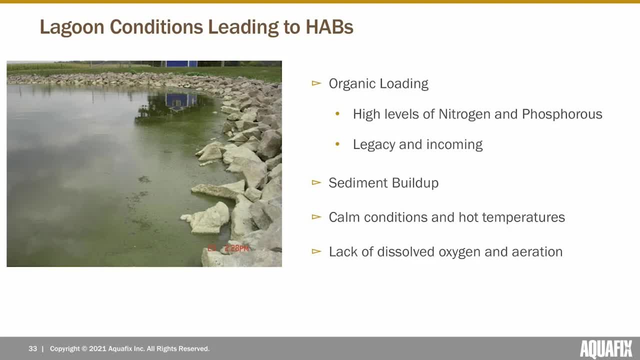 aeration can spur the opportunistic growth of cyanobacteria within your lagoon. These environmental and lagoon conditions will favor the future of the lagoon. So we're going to start with the competitive advantage of cyanobacteria over the heterotrophic bacteria, as well as your less. 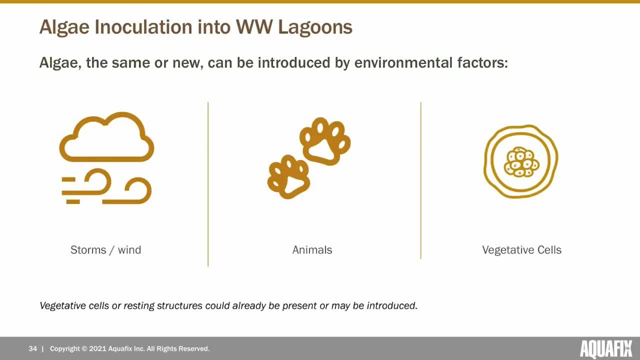 harmful green algae. New algae can be introduced into lagoons by many environmental factors. Some environmental factors include storms, wind, animals and human activities. The same environmental factors may also reintroduce an algae that you have treated previously but was now brought back into your lagoon. Some algae can also produce resting structures that may become 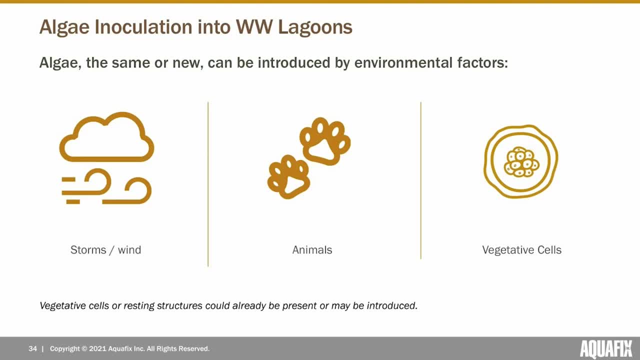 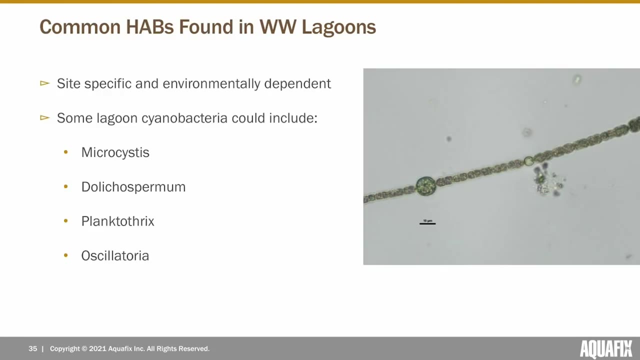 active under other conditions. Some algae can also produce resting structures that may become active under a ideal environmental conditions, And when this happens, a different type of algae may overpopulate within your lagoon quickly. This is especially likely if environmental conditions can change in favor of these vegetative cyanobacterial cells. When preparing for what types of HABs are going to, 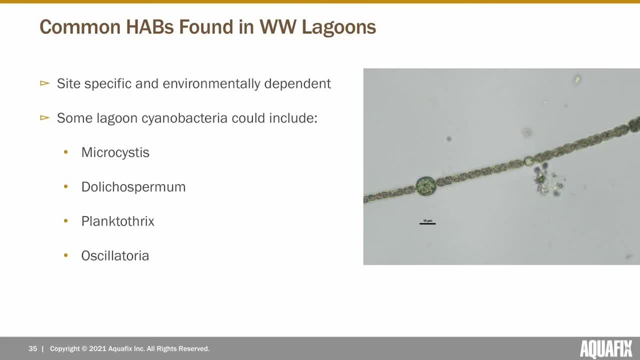 form within a particular wastewater lagoon. unfortunately, there really is no easy answer here. HAB species growth is really going to entirely be site-specific and environmentally dependent. It largely depends on the type of algae that you have. So if you have an algae that is. 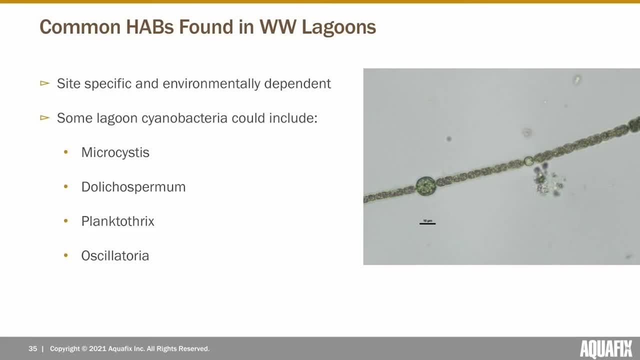 already present or inoculated within a lagoon system, as well as which HAB is most competitive in particular environmental conditions that are present. It's also going to be possible to have a mixed harmful algae bloom where multiple species are there in high abundance. Some 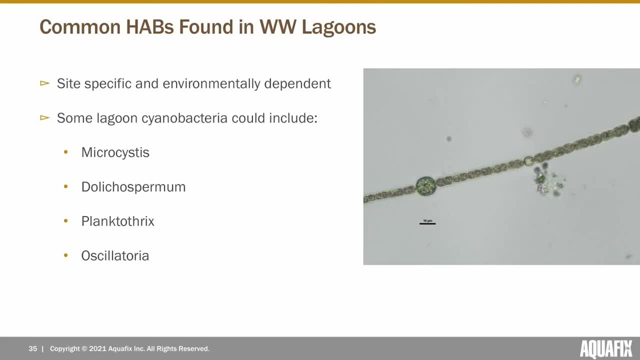 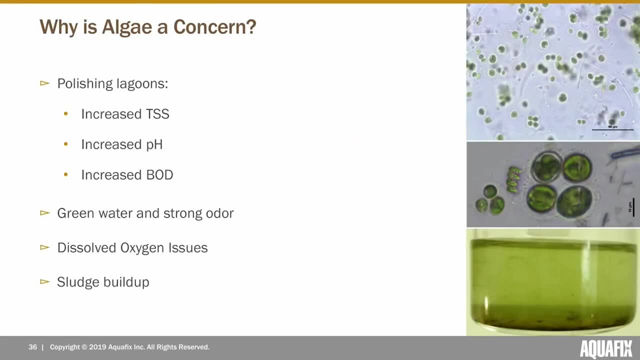 just examples of HABs that could be found in the lagoons include Microcystis Delicospernum, Planktothrix and Oscillatoria, And so in these lagoons, green algae and cyanobacterial. 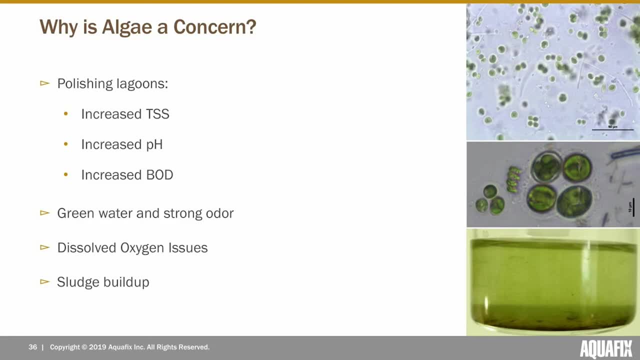 blooms can be common and they can cause many functional problems, such as increases in total suspended solids, increases in pH due to photosynthetic activity, as well as algae may increase BOD, And this is because some algae can secrete excess fixed carbon during their growth. 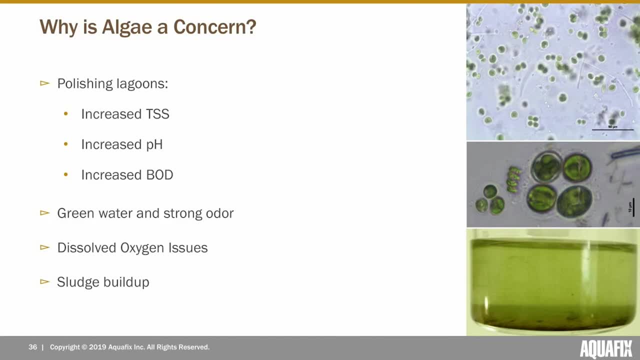 phase. Planktonic algae can also decrease the efficacy of UV or chemical sterilization from your lagoon. And finally, a bloom's presence may actually inhibit a lagoon's ability to discharge their effluent. This may mean a wastewater plant will have to use an increased 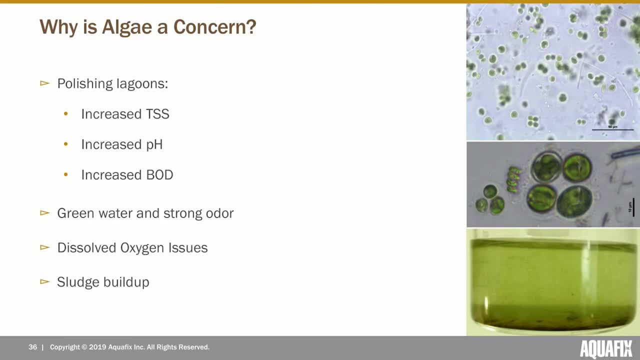 amount of chemicals or may have to extend sterilization times in order to combat the conditions within a lagoon that's experiencing a bloom. Some final concerns include green water and odor issues becoming present, dissolved oxygen issues following a bloom die-off, as well as increased sludge buildup following a bloom die-off, leading to that habitual 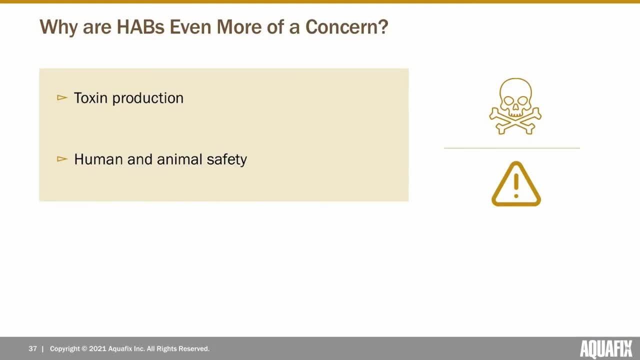 cycle, And so, although these effects of green algae cyanobacteria are very similar, HABs are even more of concern in regard to their negative side effects. This is primarily due to toxin production, and we covered the specifics of this earlier, but toxins produced within a wastewater lagoon can 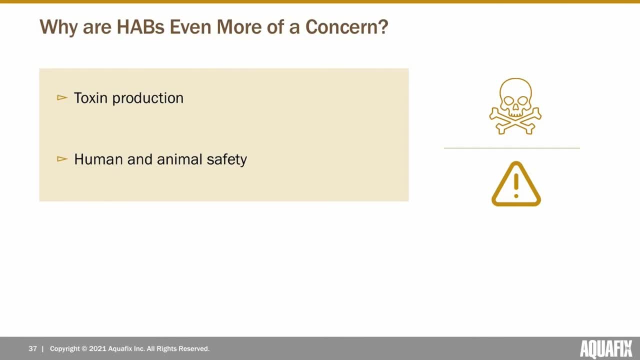 have an immediate and downstream effect. Although cyanobacteria are not guaranteed to be producing toxins, the threat of toxicity is enough for added concern due to their negative effects and impact on human and animal safety. Each year, dog and other animal deaths are due to exposure to cyanotoxins and. 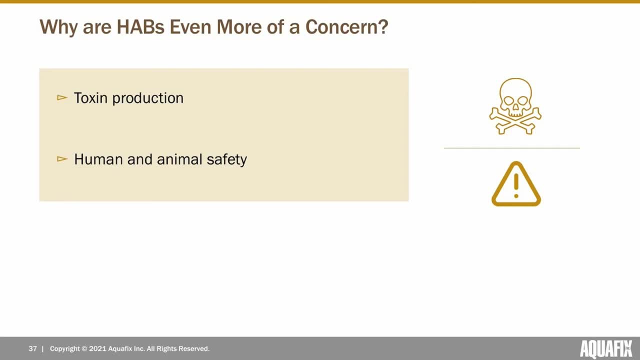 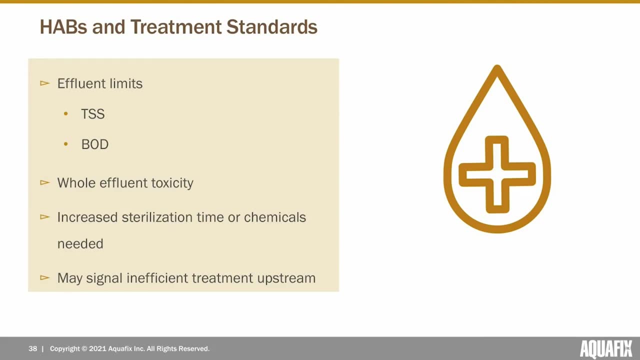 human illness can also be common when coming in contact with these toxins, And so not only are these HAB blooms potentially dangerous, they also can negatively impact a lagoons effluent standards. TSS and BOD increases from excessive algae growth can cause limit violations and lead to issues with the 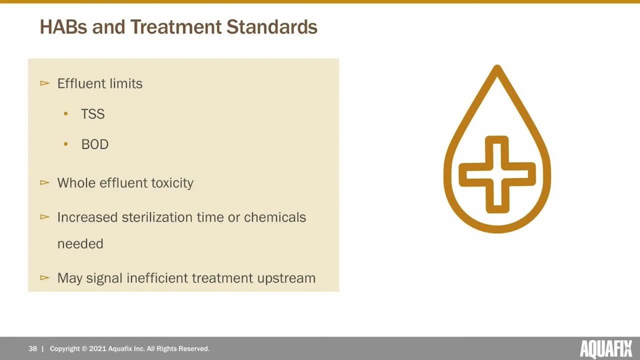 DNR and municipality. Whole effluent toxicity can also be easily failed during or after a HAB bloom, due to the likelihood of toxin release by cyanobacteria within the lagoons effluent And because of this, as I said, that increased sterilization time or 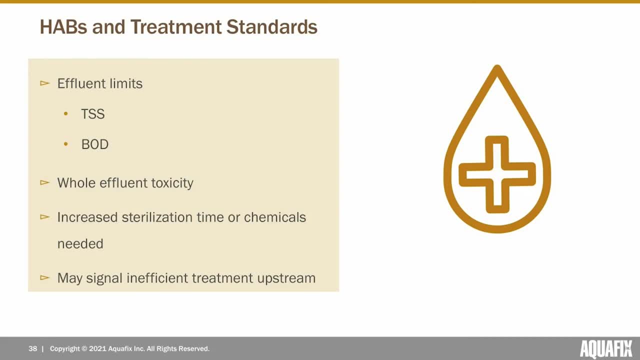 increased amounts of chemicals may be needed to maintain effluent standards from your lagoon, And also the presence of a HAB bloom may actually indicate inefficient treatment upstream within a wastewater plant or even within the lagoon itself. Overall, the presence of a HAB bloom can have a major effect on 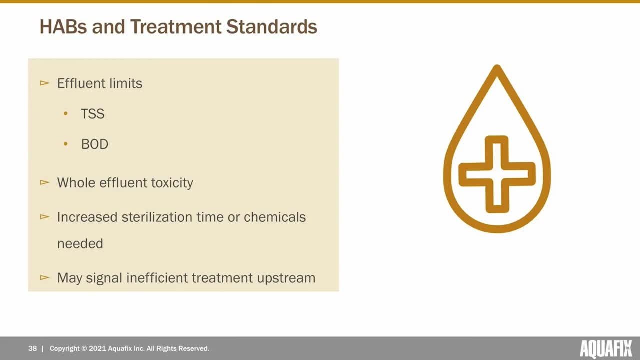 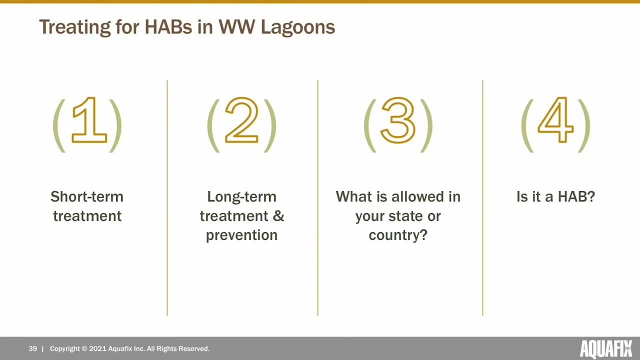 lagoon treatment standards and a number of effluent levels as a whole, And so, in order to avoid this, reactive and proactive treatment may be necessary to limit the effects of algal growth within your lagoon. There are an abundance of treatment possibilities out there, and 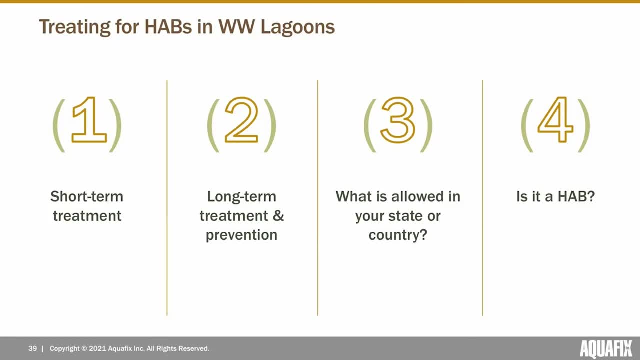 ways to try and avoid effluent limits from being broken. Our focus today is going to be on short-term and long-term treat solutions with a bacterial based focus. At the end of the day, it's important to remember that not all treatments may be allowed or may be. 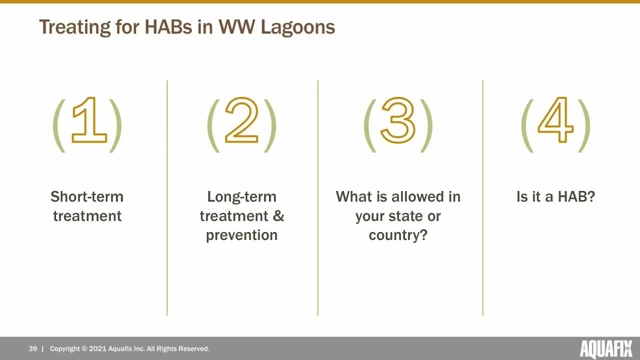 not accepted within your state or country. as well as that, it's important to identify whether or not you are dealing with green algae or cyanobacterial HABs, as treatment plans can differ between the two, As I said, for identifying what is causing your 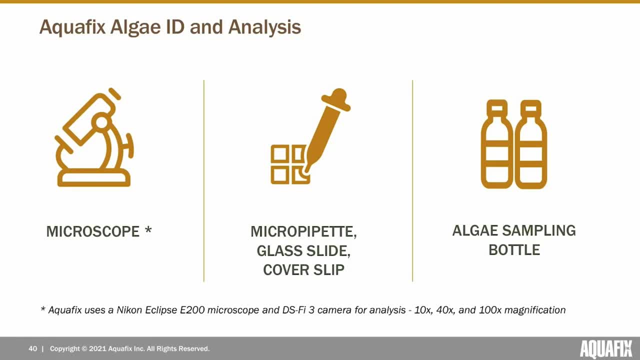 lagoon to turn green. we recommend micro analysis to identify the algae species within your bloom, whether that be a green algae or cyanobacterial based bloom. As we discussed earlier, this can be incredibly difficult to be done with the naked eye, out in the field Instead. 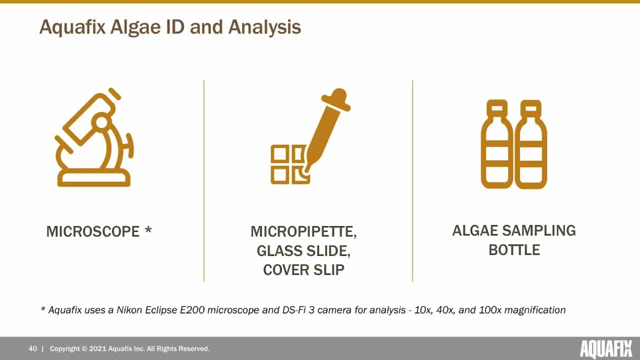 analyzing an algae sample underneath the microscope will help in the specific identification that we are looking for before beginning a treatment. Aquafix is able to provide algae ID and analysis if a sample is collected in the field and sent to our laboratory in Madison And after a correct 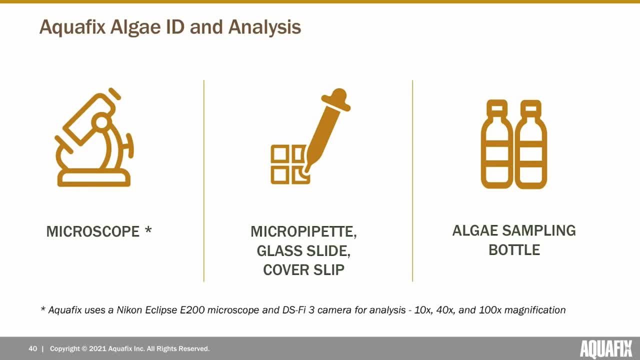 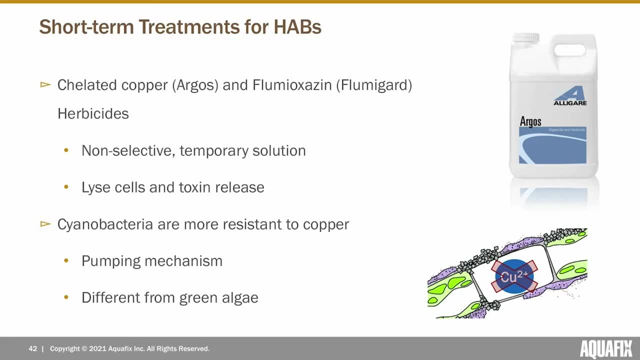 identification, we can move on to the short-term and long-term treatments. Aquafix will recommend Starting with a short-term solution. after a bloom has been formed within a lagoon, algaecides can be used to attempt to kill the cyanobacterial cells, Two algaecidal compounds. 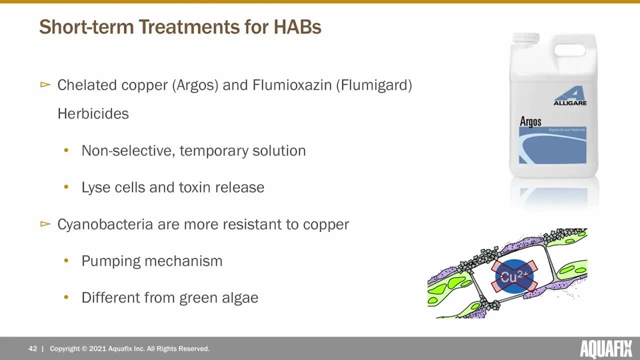 that could be effective are chelated copper, or argos, and flumioxazine or flumigard. These algaecides are non-selective and do have slightly different methods of action. The chelated copper method of action is still under debate and not entirely clear, but flumioxazine is an enzyme. 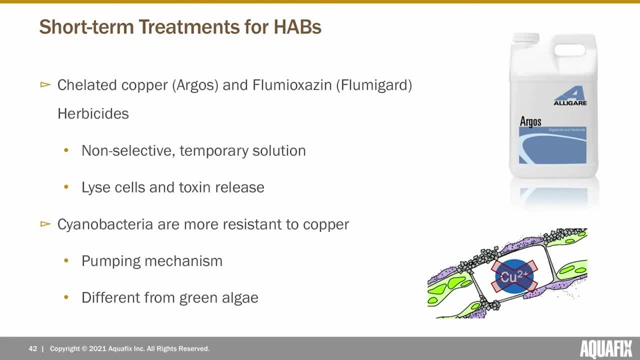 inhibitor and that can lead to allocell death. Both of these algaecides are temporary solutions, as they only induce cell death and are relatively short-lived treatments. These short-term treatments can end up releasing more toxins, as cyanobacterial cells lyse and the 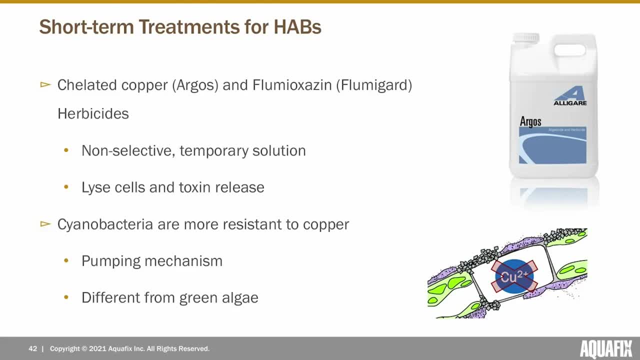 toxin is thus released into the lagoon water. One other note about these algaecides is that cyanobacteria are often actually more resistant to copper in comparison to green algae, And this is because cyanobacteria are fundamentally different from green algae on a cellular level. 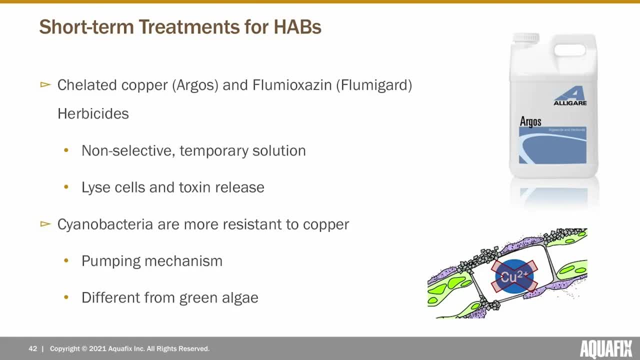 and also have a metal pumping system that can effectively pump out the cyanobacteria from the algaecide. So if you have a cyanobacteria, that is copper out of cyanobacteria cells prior to cell death due to that copper molecule. 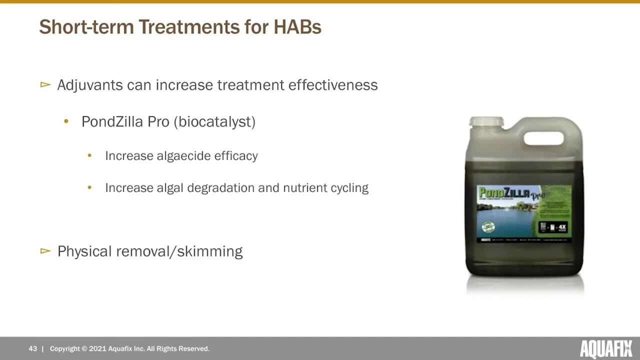 In order to make these algaecidal treatments more effective on cyanobacteria, Aquafix has additional short-term treatment solutions that can increase algaecide effectiveness as well as increase the amount of time between bloom occurrences within a troubled water body. 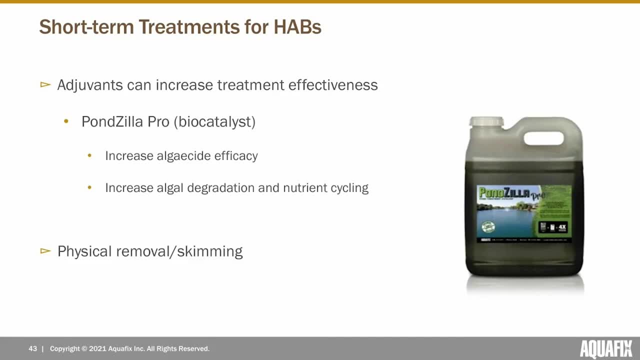 Our adjuvants can be used to provide a synergistic effect with algaecides. Ponzilla Pro- here is a biocatalyst that can help increase algaecidal penetration, as well as increase algal cell degradation during and after an effective algaecidal treatment. This can help clarify. 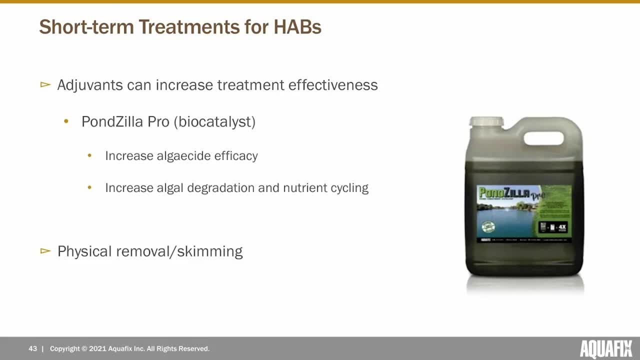 the water column, as well as limit the amount of dead algal cells settling into the sludge layer. due to Ponzilla's ability to degrade dead algal cells as well as their contents, Less nutrient release and possibly less toxin release after an algaecidal treatment will really be able to be. 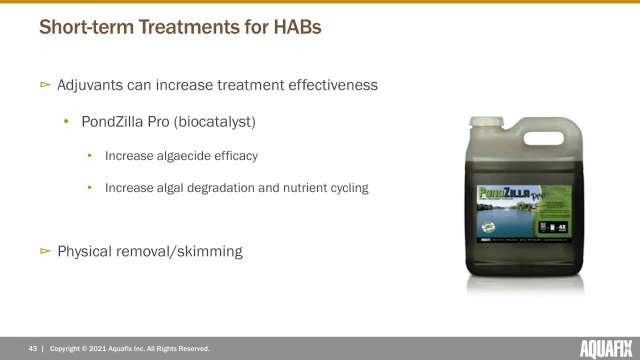 a goal and a help with these treatments. Also, physical removal and skimming of the algal cells during before, during and after an algaecidal treatment will also help with removing some of those nutrients out of the water body and restricting some of 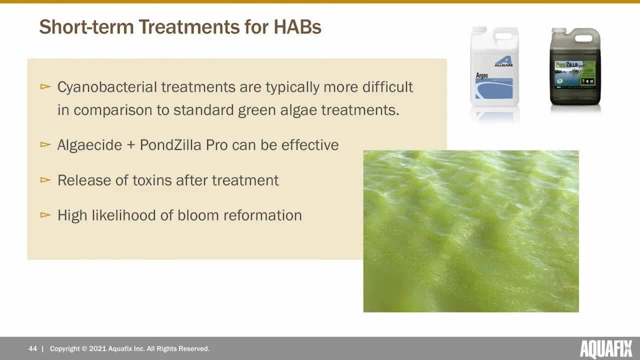 that sludge buildup from occurring. So overall, it's important to understand these takeaways in regard to short-term HAB treatments within your lagoon. First cyanobacterial cells: First cyanobacterial treatments are typically more difficult in comparison to your standard green. 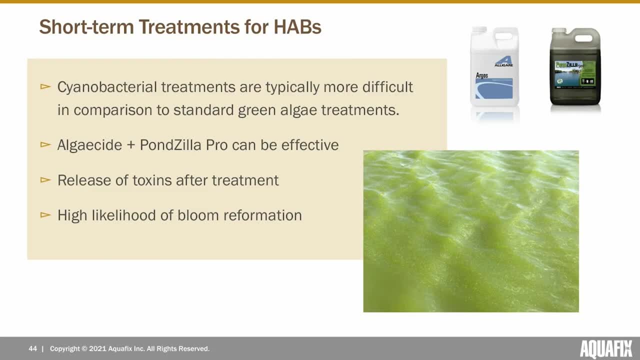 treatments due to differences in morphology, As we were dealing with photosynthesizing bacteria, not green algae. Although applying an algaecide in Ponzilla Pro can be effective in killing off a HAB bloom, there are some unintended negative side effects to 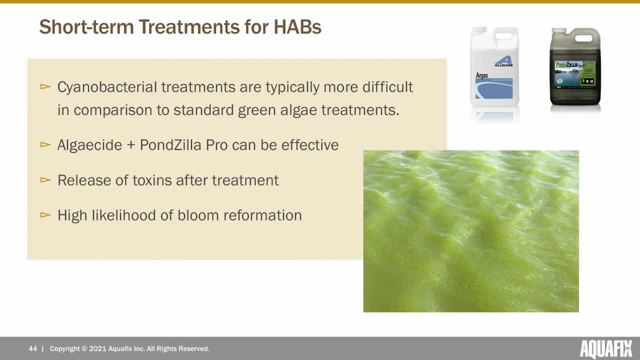 short-term treatments. First, as I said, toxins can be released after HAB cell death, which can cause issues in regard to effluent standards and animal health. Also, while focusing on short-term treatments, although the bloom may disappear, there really is a strong likelihood that bloom 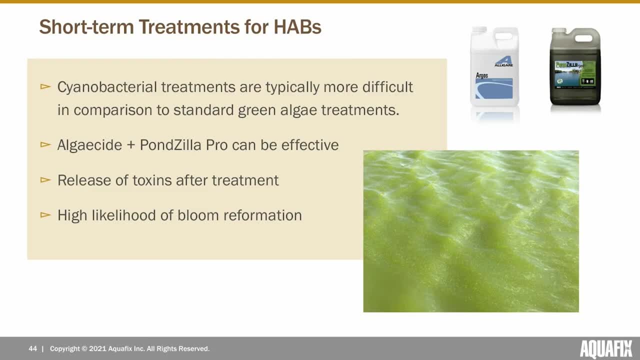 reformation may occur due to environmental conditions, So if you're looking for a short-term treatment, you may want to consider a long-term treatment that supports HAB growth. Because of this, long-term proactive treatments may be necessary and are the preferred solution. 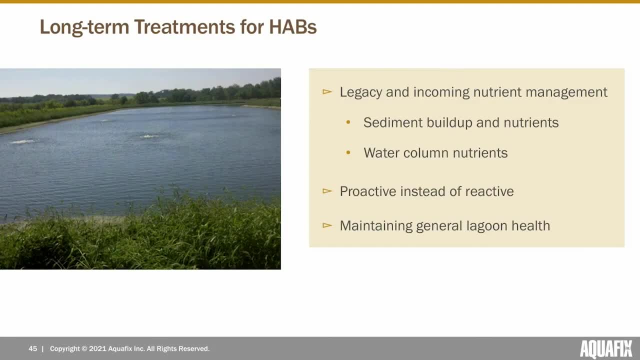 So, regarding these long-term treatments, we are going to discuss proactive management strategies designed to combat the legacy and incoming nutrients within a wastewater lagoon, as these are really fueling that cyanobacterial growth. This is going to be both within the sediment. 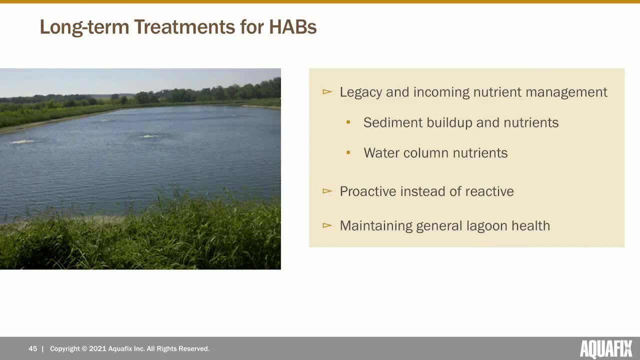 as well as the water column. And, as I stated, these strategies are proactive, effective measures that are going to try and maintain general lagoon health as well as limit harmful algae growth occurrences within your lagoon. The proactive strategies that I'm going 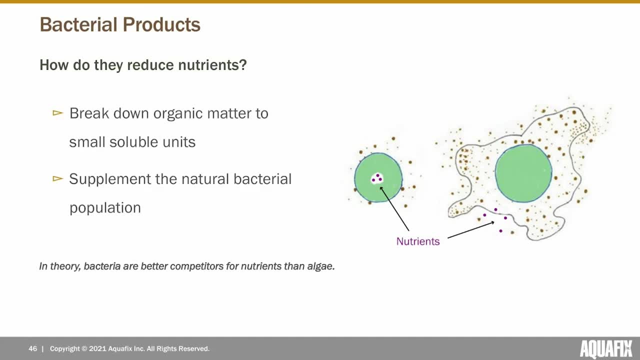 to be discussing are going to be bacterial-based, And so I'd like to take a second to discuss the science behind bacterial products and reducing nutrients. Bacterial-based probiotic products are a combination of bacteria and select stimulants in order to not only introduce 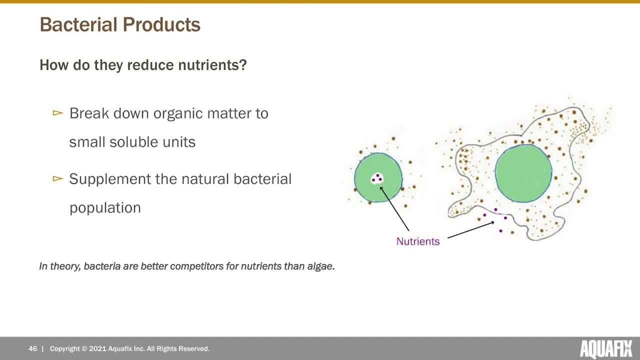 and activate new heterotrophic bacteria, but also stimulate and supplement the natural bacteria population that's already going to be present within a wastewater lagoon system. The goal of these products is to help reduce incoming nutrients and the internal nutrient reservoir within the lagoon through the breakdown of 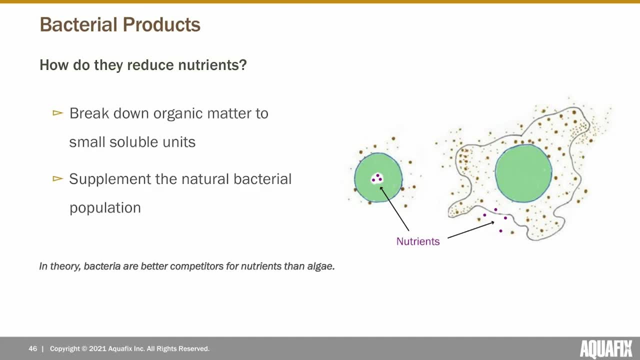 organic matter into smaller soluble and usable units. Bacteria are much smaller than algae and because of this have a much higher surface area to volume ratio, And because of that in theory this should make bacteria much better competitors for these soluble nutrients in comparison to the larger algal cells. 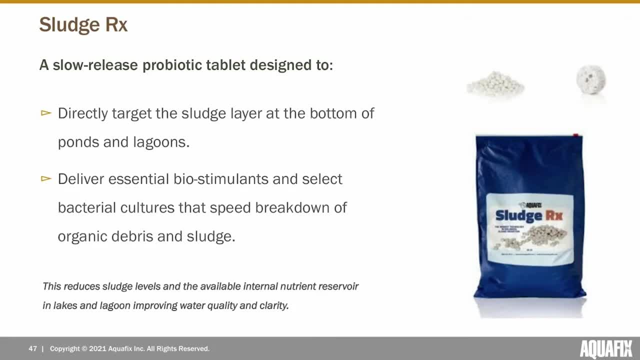 The first probiotic product I want to discuss is SludgeRx. SludgeRx is a slow-release tablet containing bacteria and stimulants that was designed to sink directly and target the sludge layer of a water body or wastewater lagoon. The application of these stimulants and bacterial 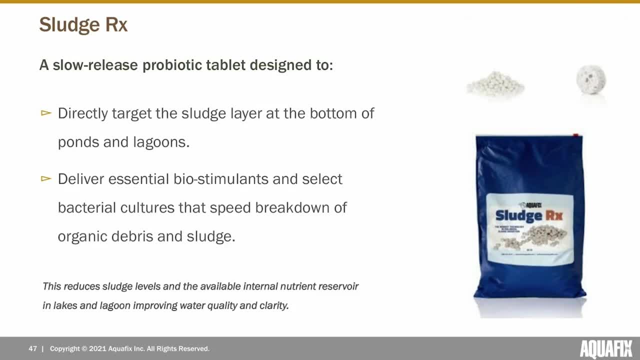 cultures is intended to increase bacterial activity and metabolism and thus speed the breakdown of the organic sludge that is present in the sludge. This is a product that is used to increase bacterial activity and metabolism and thus speed the breakdown of the organic sludge that is present in the sludge. 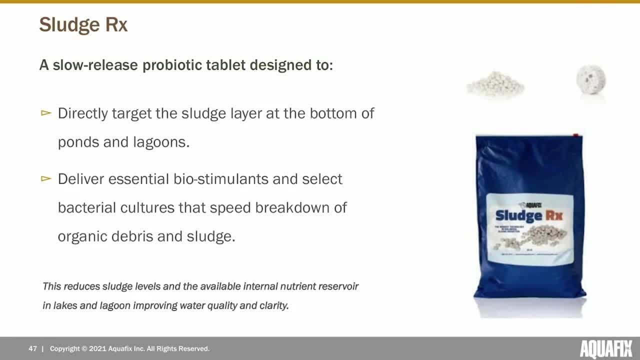 This will not only reduce the overall sludge level within the lagoon, but through the breakdown of the organic sludge, the sludge material, will reduce the nutrient reservoir within the sludge. Because of this, water quality and clarity should increase with a. 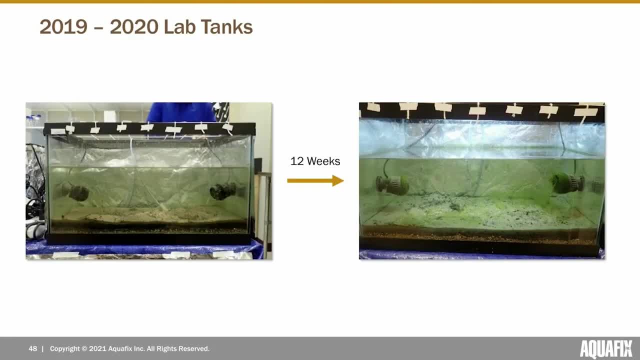 larger amount of sludge in the lagoon. To test our ability to reduce sludge and nutrients, we have designed a testing method that uses using these 15-gallon aquarium tanks with two side bumps that generated lateral water movement. We also had an aerator in the middle of these tanks that was able to provide aeration as well. 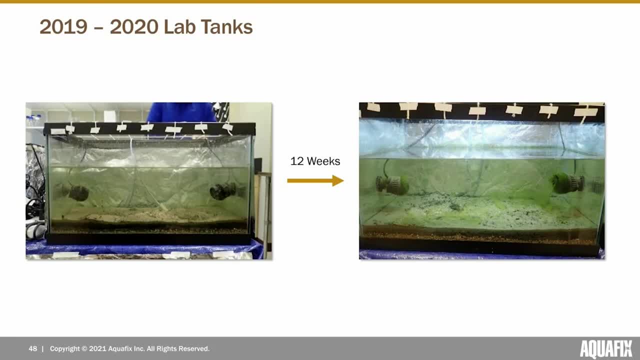 as some limited vertical water movement within the tanks. The tanks were wrapped in foil in order to prevent differences in light exposure and the only light in each tank was a fluorescent fish tank grow light that was set on a 12 to 12 light and dark cycle. They were within the actual tank. 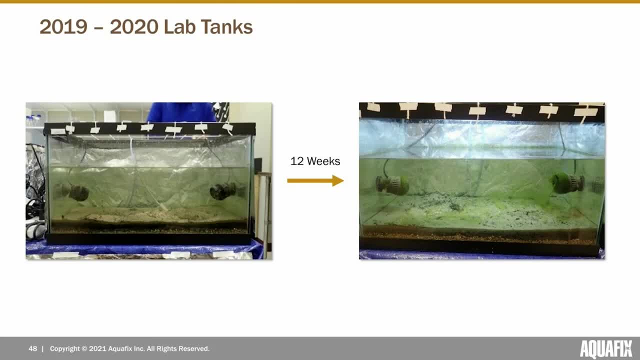 At the sediment layer we had a bottom two centimeter layer of sand on the very bottom. On top of the sand layer we had a half centimeter wash clay layer and then on top we had two centimeters of pond sediment. These tanks were then filled with pond water to a height of 15. 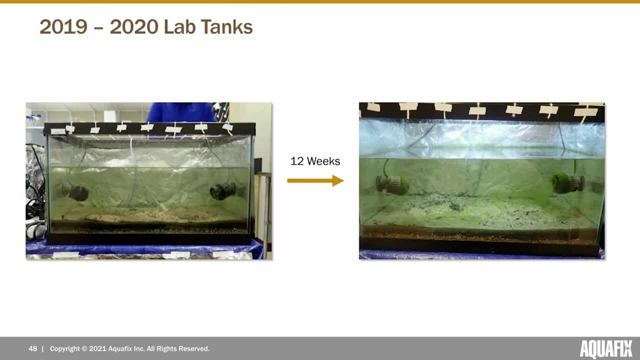 centimeters above the sediment layer, and the tanks were dosed with 12 and a half pounds per acre of sludge RX every month for a three-month duration. Sediment depth was measured weekly in these tanks using 30 different quadrants to measure an overall sediment depth and measurements. 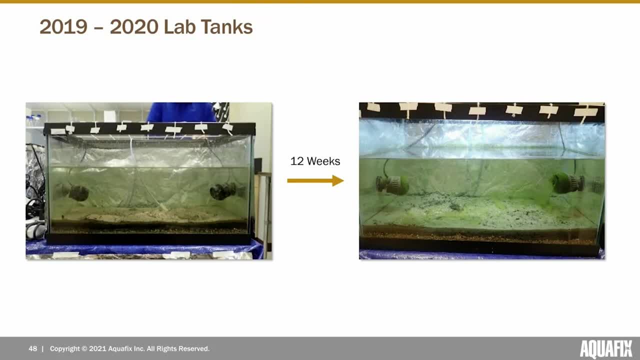 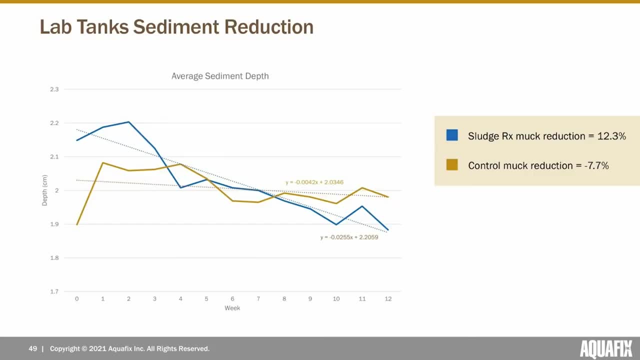 of sediment nutrients were also taken before and after the 12 weeks of testing. So I'd like to discuss some of the data from this experiment now. So first we can take a look at the sediment reduction that occurred within these test tanks after being applied sludge RX, As you can see in: 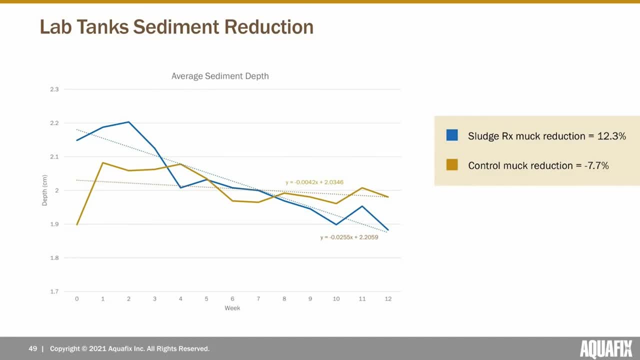 the blue line. there we have a nice good negative trend line of sludge reduction throughout the entire experiment and we were able to see sludge reduction occur with the application of sludge RX. We compare that to control tanks where we really did not see. 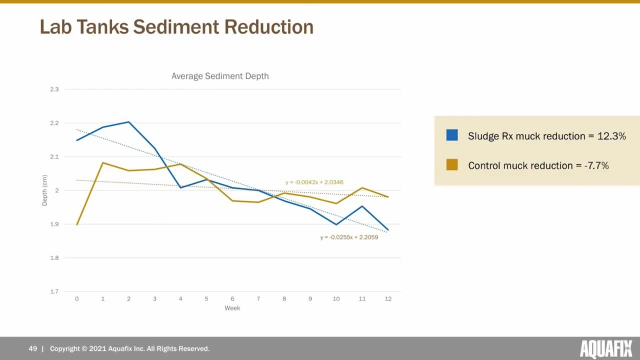 much sludge reduction or much sludge increase, but we kind of saw relatively stable levels throughout the entire experiment. So we were happy to be able to see sludge reduction and we've been able to prove this many times throughout similar experiments to this. As I said, after 12 weeks of 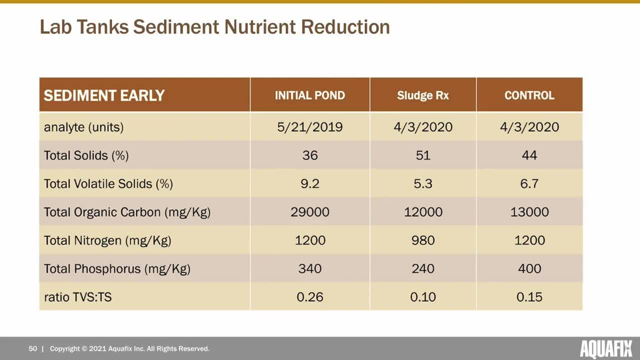 testing of applying sludge RX. we were able to see sludge reduction and we were able to see sludge reduction and we were able to see sludge reduction. as well as control tanks. We measured and averaged out your sediment nutrients that were still present. The sludge RX tank had. 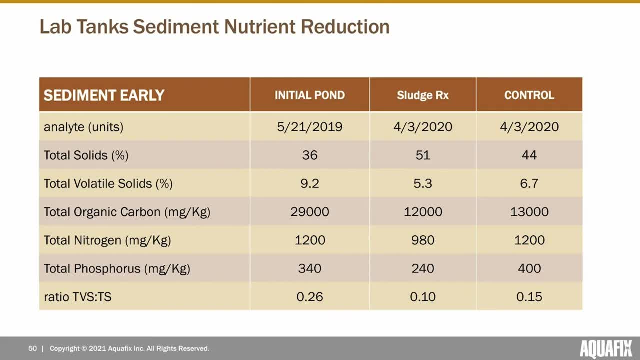 higher levels of total solids and lower levels of total volatile solids in comparison to the control tank and the initial pond muck. The sludge RX tank also had lower levels of total organic carbon, total nitrogen and total phosphorus in comparison to the control tank. after 12 weeks of testing, We were happy to see less. 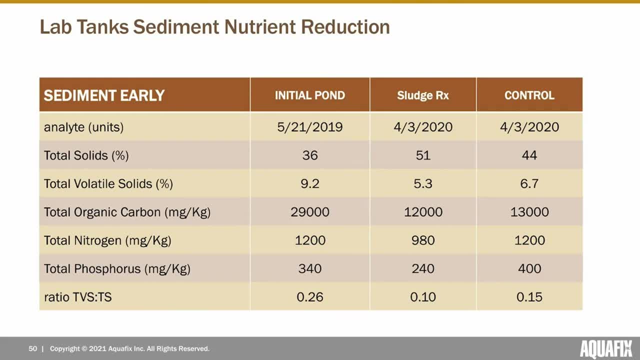 nutrients still present within this tank, andacao. underground substances were removed and we were able to sixteen days after this test tank. And when we talk about total solids and total volatile solids- as I'm sure most of you know, when we're talking about that, the measurement for total solids is determined from filtering. 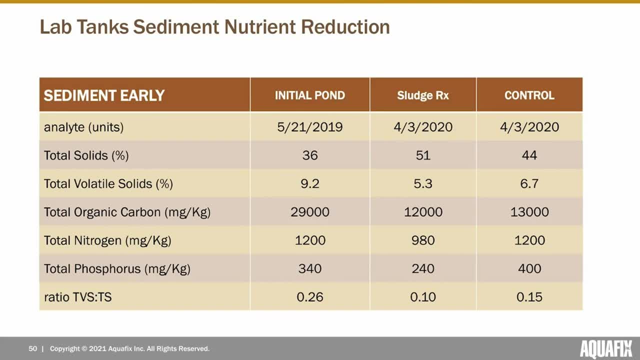 your sediment onto a 1.5 micrometer pore filter, drying that filter and weighing it. Then, after you weigh it, burning that filter in a furnace and weighing it again. The amount of solids that are burned off of that filter are going to be your total volatile solids and are going to be 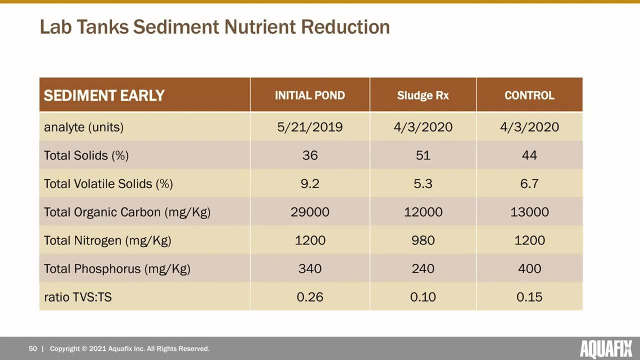 considered the organic portion of your sediments. We like to look at the amount of total volatile solids as the amount of organic sediment that we actually are able to break down biologically and able to reduce those nutrients through that breakdown process. So at the end of the 12 weeks, 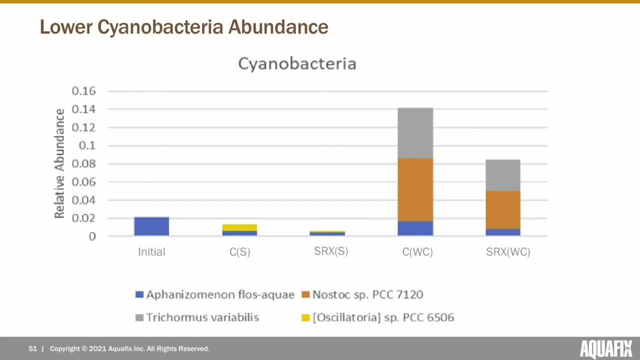 we also sent out the sediment and the water for metagenomic analysis And we looked at all the DNA in both the water column and the sediments. One thing that was interesting is when we looked at the DNA of cyanobacteria Between our tanks that had SludgeRx applied and our tanks that were acted as controls and had no 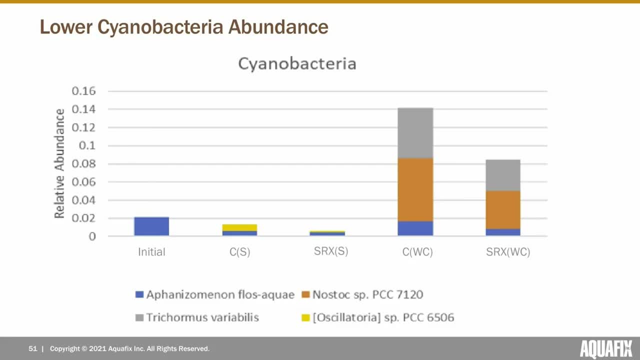 application, we saw that there was much higher levels of cyanobacteria present within our control tanks. If you look at this graph, you see our initial levels of cyanobacteria within the initial pond sediment And then we have our control sediment, our SludgeRx sediment and then our 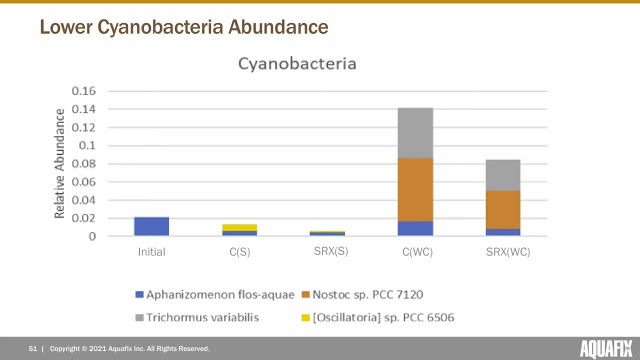 control water column and SludgeRx water column- relative abundances of cyanobacteria present. As you can see, we have a lot of cyanobacteria present. We have a lot of cyanobacteria present. As you can see, there was much more cyanobacteria found within the water column in comparison to the 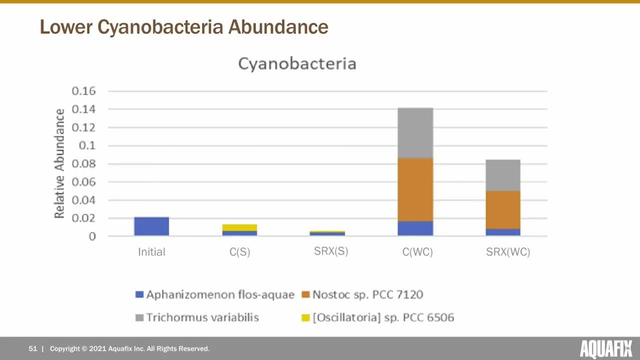 sediment in general, And this is most likely due to cyanobacterial cells that were present within the sediment at the beginning of testing, being able to control their buoyancy and float into the water column as growth conditions began to be optimal for those cells. But at the end of the 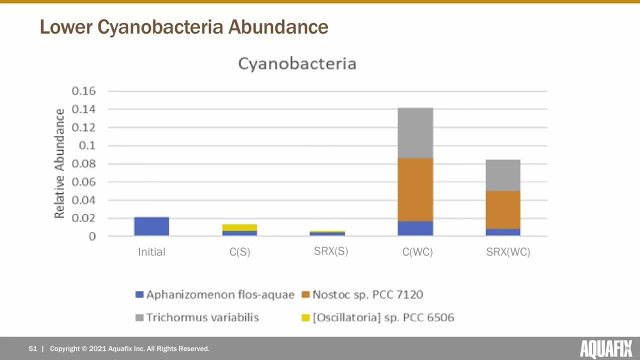 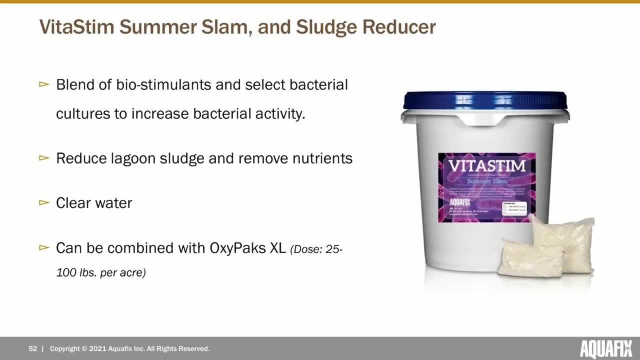 day. what we were able to see was that the tanks that were treated with SludgeRx did end up having lower levels of cyanobacteria. So I'd now like to discuss another probiotic product that we can provide, which is more targeted for the water column rather than the Sludge layer like SludgeRx, as we just discussed. 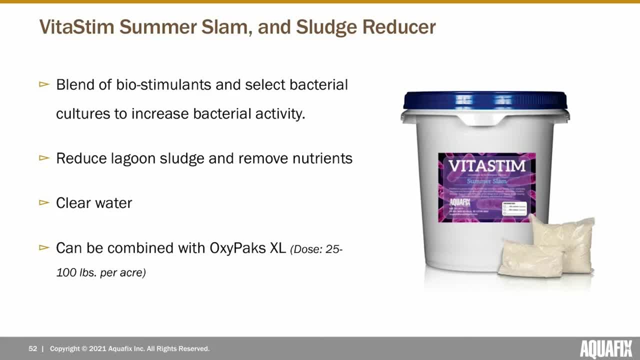 What I'm talking about here is VitaStim, SummerSlam and SludgeReducer, as they are specific powdered blends of biostimulants and select bacterial cultures that are designed to grow within a lagoon and pond and reduce sludge and nutrients. This not only clarifies the water, but also the 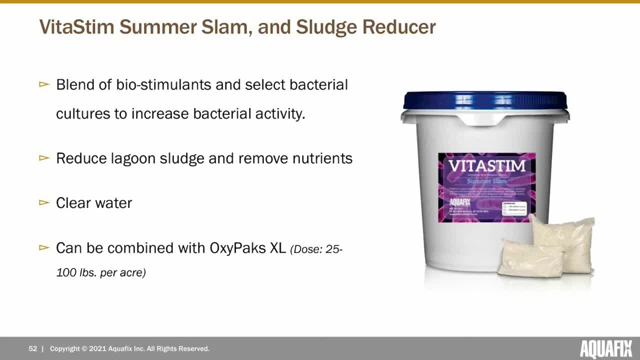 bacteria that are present within the lagoon. It also can be used after a copper treatment in order to restore your bacterial health within your lagoon. VitaStim SummerSlam and SludgeReducer can be combined with Oxipax XL, which can be used to boost oxygen levels and float softer bound. 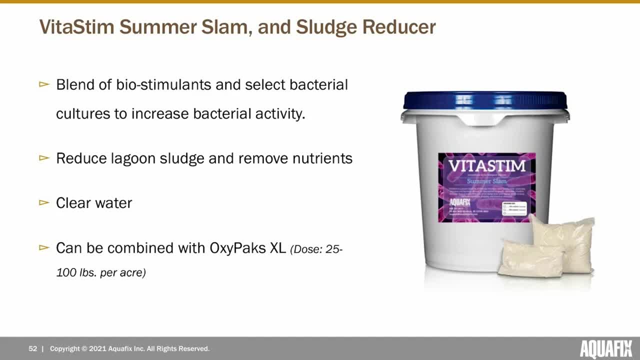 sediments into the water column, which can be broken down quickly by SummerSlam and other bacteria that are present. Overall, the proactive probiotic treatments that I'm showing here, both for the water column and for the sediment, should help reduce occurrences of harmful algae. 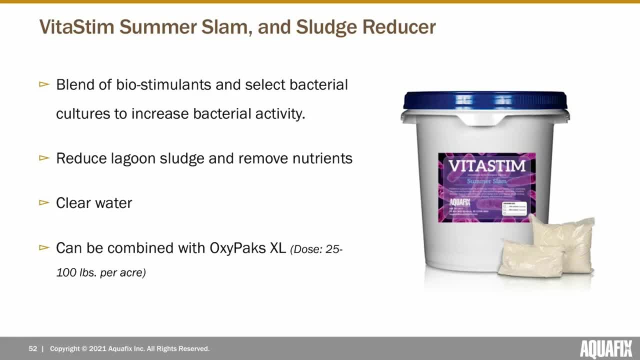 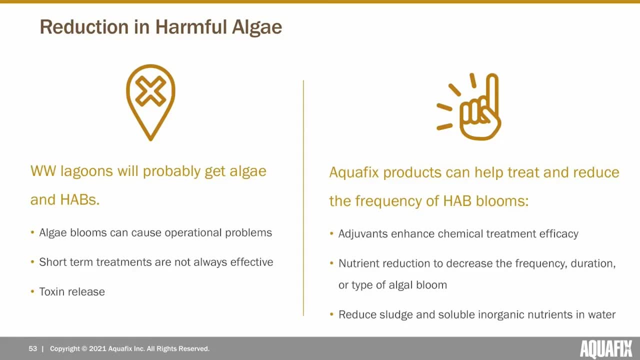 as our products are attacking that internal nutrient reservoir and trying to bring back a balanced and healthy community in your wastewater lagoons. And so to kind of summarize that point in trying to get this reduction in harmful algae, unfortunately, the way wastewater lagoons are, 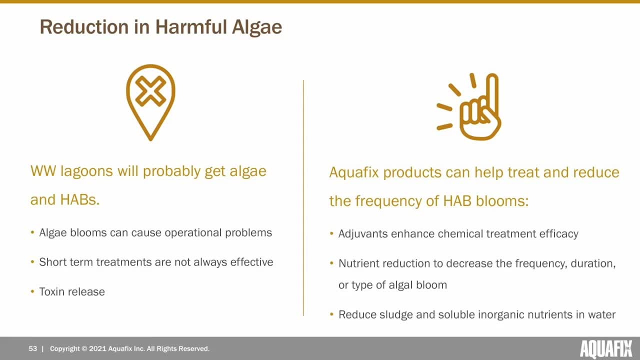 constructed and fed with nutrients, they probably are going to get- whether it be algae or harmful algae, at some point during their life cycle. Algae blooms can cause these operational problems, as we discussed Today, and short-term treatments, although they can be effective, are not always going to be. 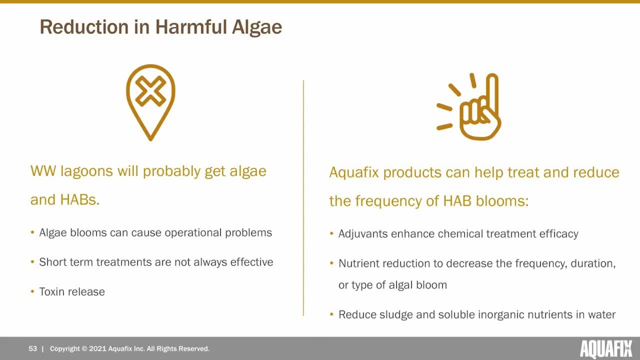 effective and can actually lead to bloom formation reoccurring due to it not being a long-term solution. The other issue with these short-term treatments is that toxin release, as I had said earlier, from cell lysis after a treatment. But through our research and through our solutions. 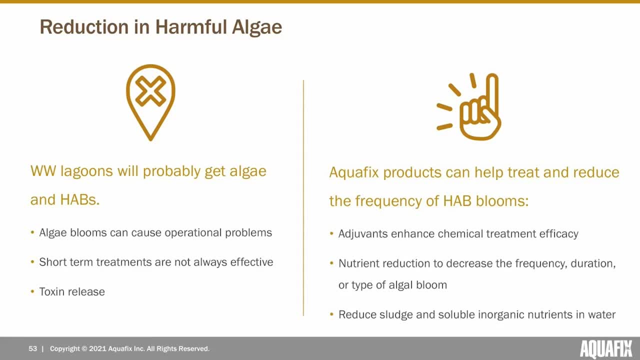 we believe that our Aquafix products can help treat and reduce the frequency of HAB blooms proliferating within your lagoon. Our adjuvants can help enhance chemical treatment efficacy and enhance the amount of time between necessary chemical treatments, as well as our probiotic products can help in the nutrient. 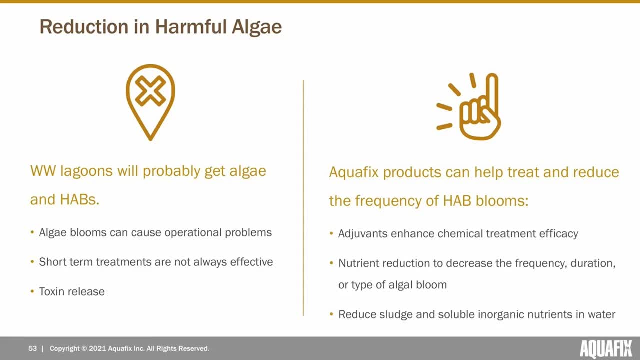 reduction of the internal nutrient reservoir of a wastewater lagoon And this can help decrease the frequency, duration or type of algae bloom. And our whole goal is to reduce that sludge and reduce the amount of soluble inorganic nutrients within the water column in order to not only make 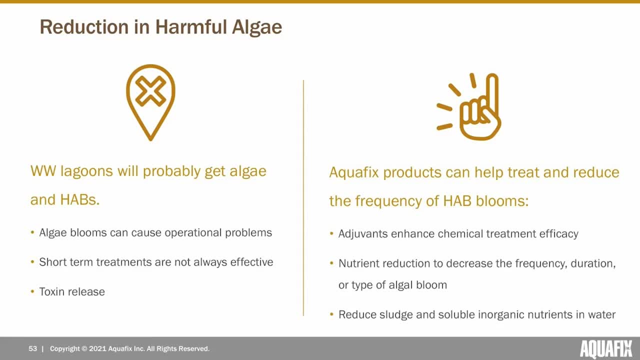 a healthier lagoon environment, but also reduce the amount of soluble inorganic nutrients within the water column, in order to not only make a healthier lagoon environment, but also reduce the ließen, its energy, as well as control and live in a fresh, smooth, clean, resilient climate. 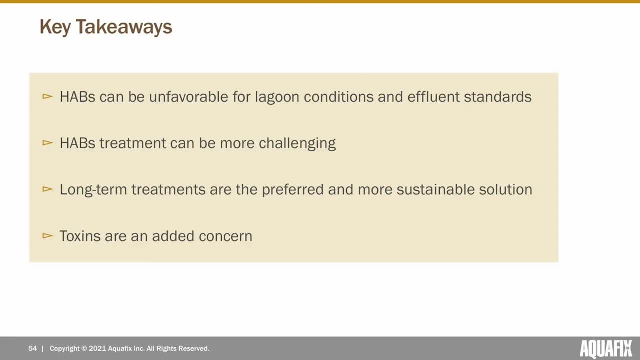 Die. now some final key takeaways from this presentation as a whole. I just want to remind everyone that, as we expect HAB growth to continue to increase in the future, HABs' can be unfavorable for lagoon conditions as well as your effluent standardsThe treatment of HABs. 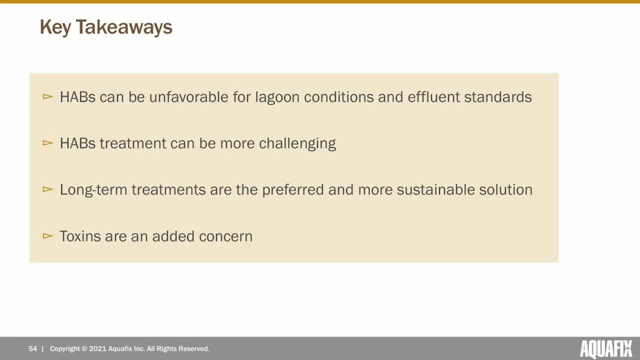 can be more challenging than the treatment of your standard green algae within a lagoon system. and long-term treatments and really going after that nutrient reservoir is going to be the preferred and most Independant informed treatment of aquaculture or phone and interessant exegetics. 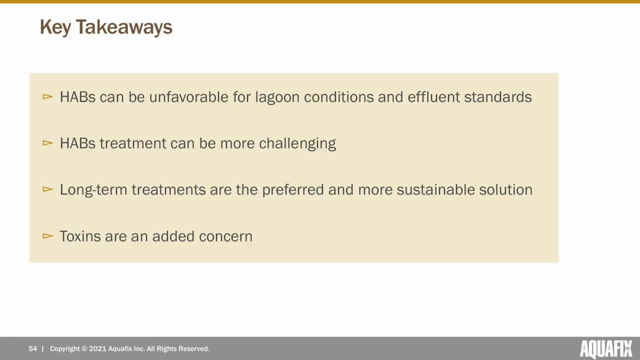 more sustainable solution With HAV specifically. as I've reiterated throughout this presentation, the toxins are going to be an added concern, And that's something that we always have to be aware of in order to protect human and animal health, And with that, I'd just like to remind all of you. 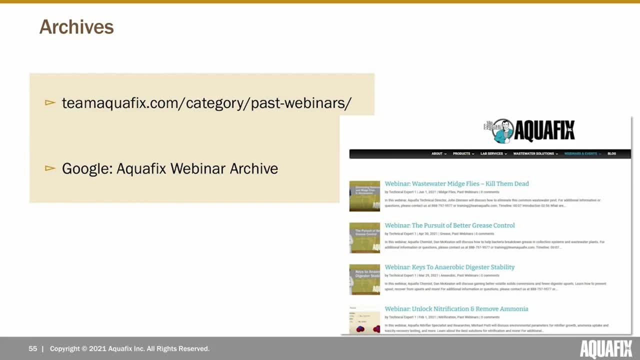 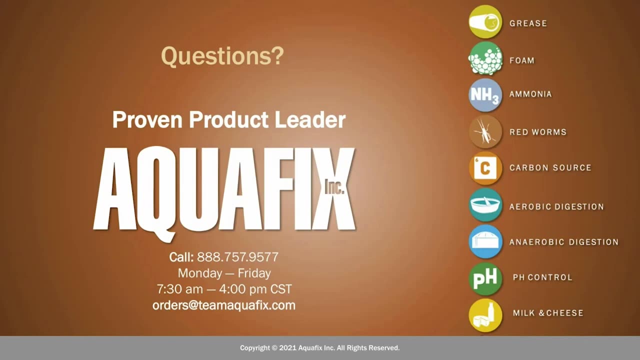 here today that all of our webinars done by the Aquafix lab and team can be found online on our website and our Aquafix webinar archive. You can go there to see any of our previous webinars, And here actually is a link as well to go directly there. And with that I'd like to open. 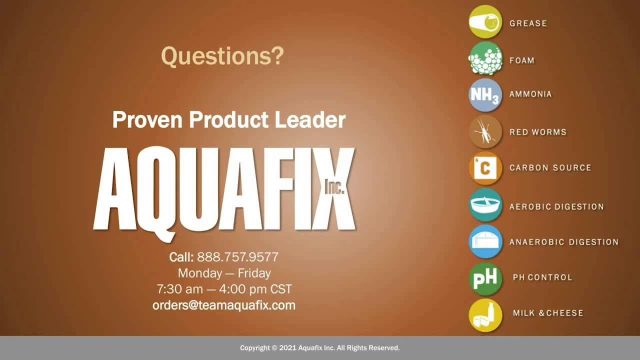 it up for any other questions that anyone has. I see one here from David about what do you have to treat algae if I cannot use copper products? Well, it's tough And I know a lot of times copper products cannot be allowed or are highly regulated in specific areas And I guess my biggest 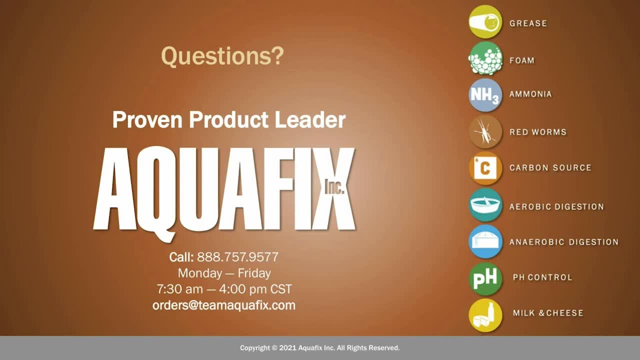 recommendation in that would be to get ahead and try and reduce the amount of algae that can be growing And that's going to be really important And I'd like to see a lot of people in the those probiotic solutions and trying to maintain lagoon health in order to not favor the growth of 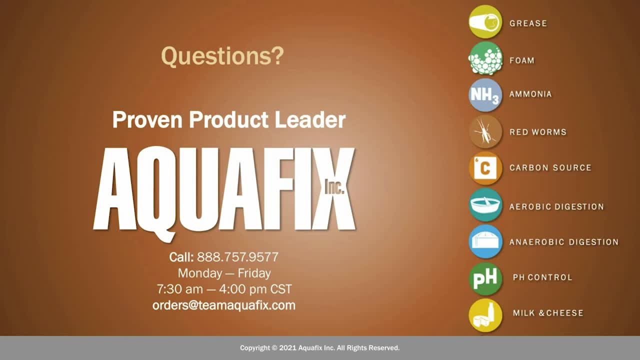 green algae and cyanobacteria. And here's a question from John- And would you say most problems in wastewater lagoons are traced back to the sludge layer as a root cause? And, yeah, I think that is a fair message to provide as these lagoons the way they're set. 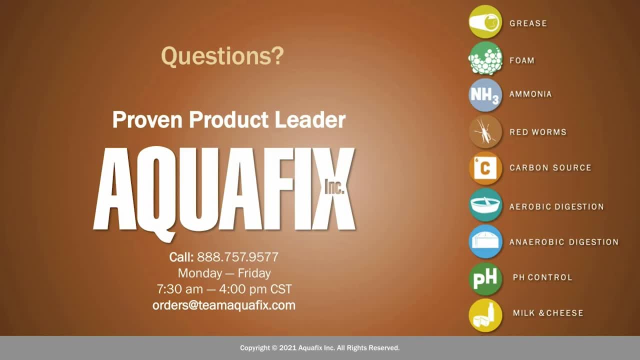 up with the amount of solids and nutrients coming in, you're going to get this buildup of sludge And, as we discussed in today's webinar, that buildup of sludge is going to lead to a higher levels of nutrient release internally into the lagoon And that internal release of nutrients 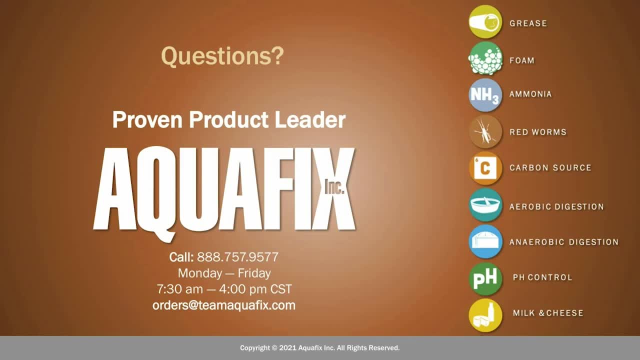 from that sludge layer can really just fuel these not only algae growth but also harmful algae growth. And really being able to attack that sludge layer should be the first line of defense against algae growth within your lagoon, as we can try and reduce the amount of sludge present. 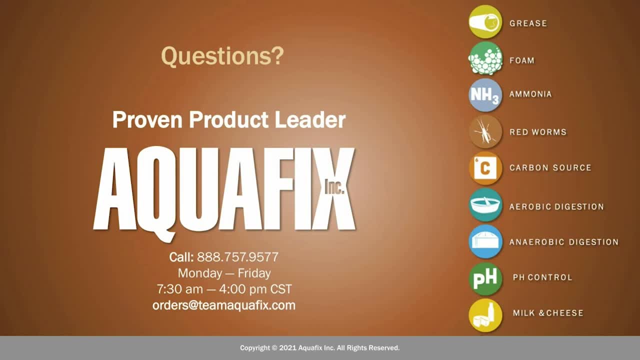 as well as reduce the amount of nutrients. within that, It could be fair to say that most, most problems can be traced back to a buildup of sludge leading to algae growth within lagoons. So this question here: use of copper can eventually cause 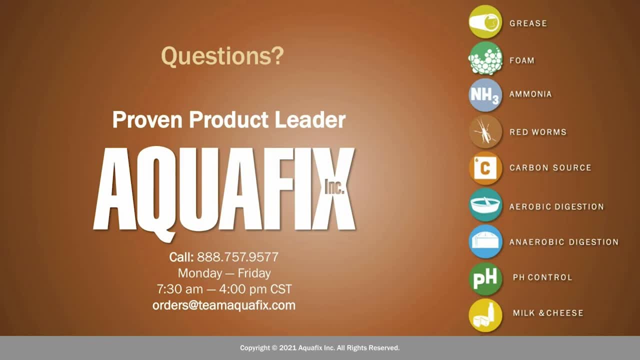 problems for sludge accumulation. I agree as you can. all these cells can end up settling down into the sludge and asking if the aquafix products can accumulate in the sludge. And so, as you are applying these tablets into the sludge layer, they are not in sense leading towards these. 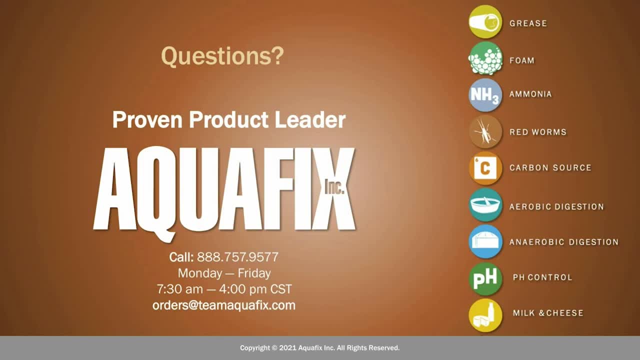 larger algal cells accumulating within the sludge, as these bacterial cells within these aquafix products are going to be trying to break down and digest that sludge and remove sludge. So although you are adding a product into that sludge layer, that product is looking at the benefit of trying. 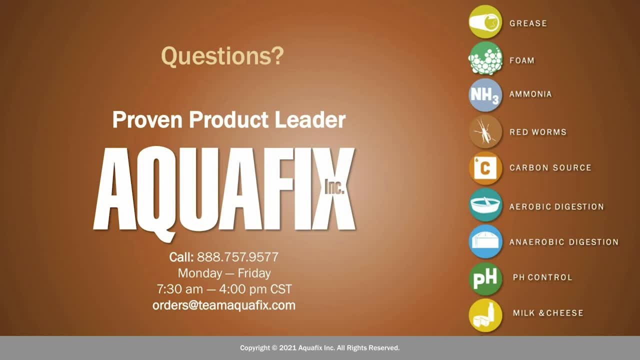 to reduce and remove that sludge from the wastewater lagoon rather than accumulating it, like these larger algal cells and these large organic sediments And or aquatic plants, for example. But I don't see any other questions If anyone does have. 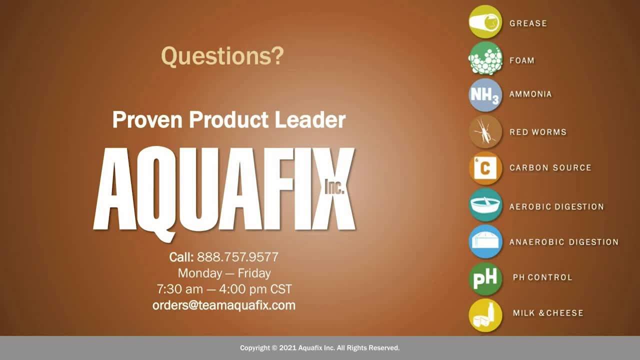 any questions. feel free to email and reach out to aquafix and any of us at any time And we can be there for a call or for an email or anything to respond, to try and help out and be a partner in combating any algae that's growing within your wastewater lagoon. But I just would like to thank 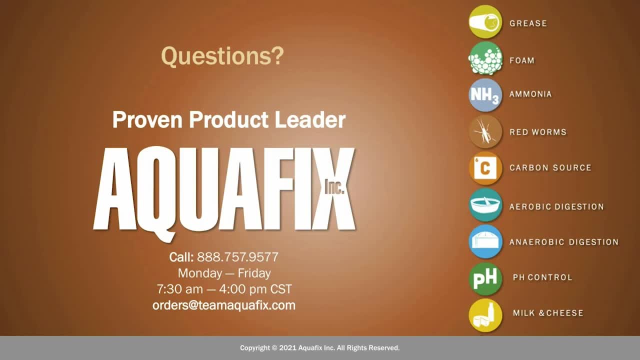 everyone again for joining us today. I really appreciated the time and being able to present And again, we are open. We're always here for help. if anyone has any other questions and just let us know and we will be there for you. Thank you, Hope everyone has a great day and appreciate it.